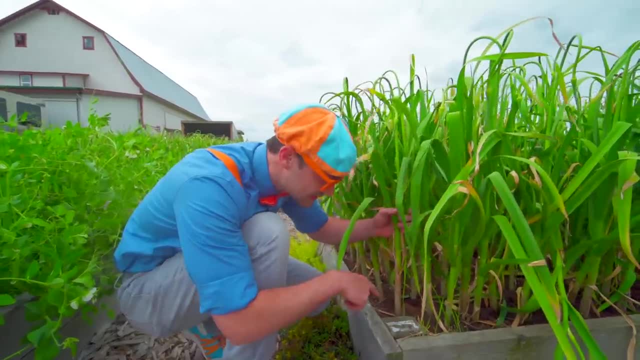 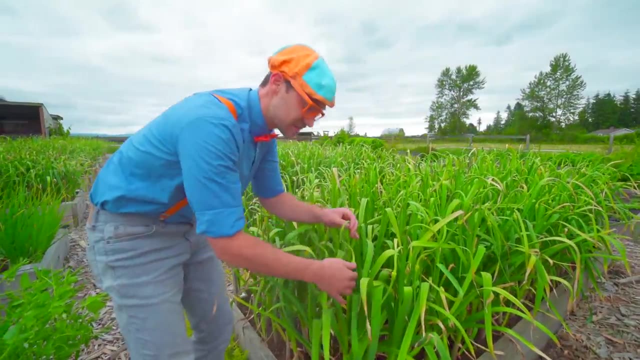 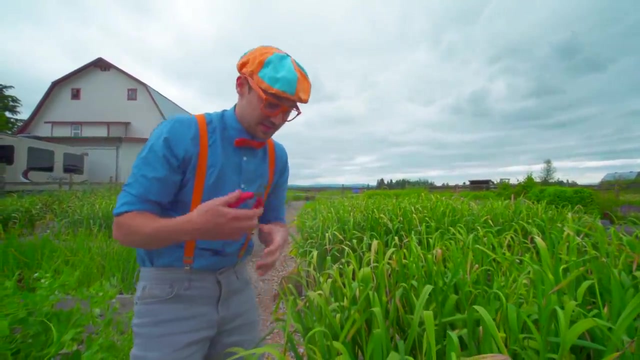 So garlic is actually a bulb right down there, But it's not ready to be harvested yet. But up here you can harvest the tops, And it's also tasty. I'll show you how to do that. So I'm going to take these really sharp scissors, So I'm going to be very careful. 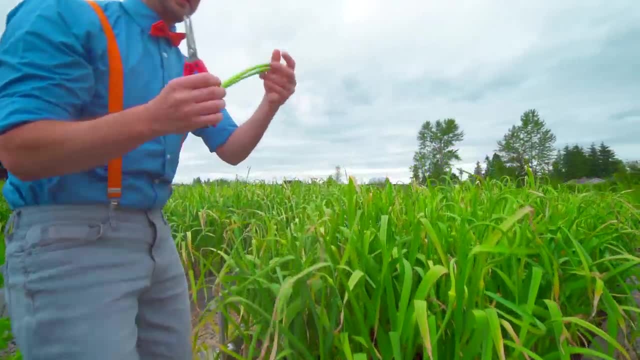 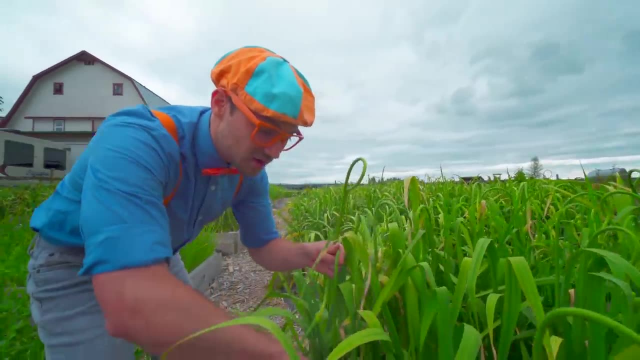 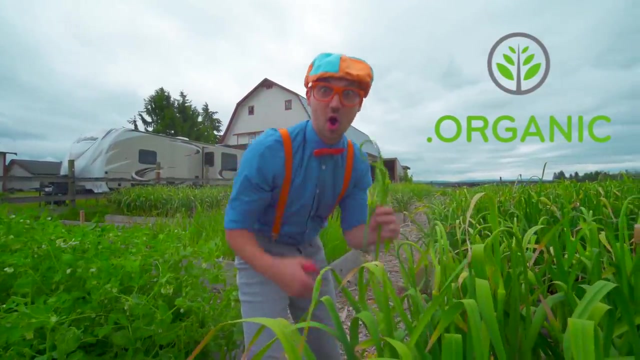 And I'm going to snip it right there. This is what it looks like: Whoa. One great thing about this farm is that all the food and the flowers are organically grown. This is going to be so tasty. All right, I think that's good enough. 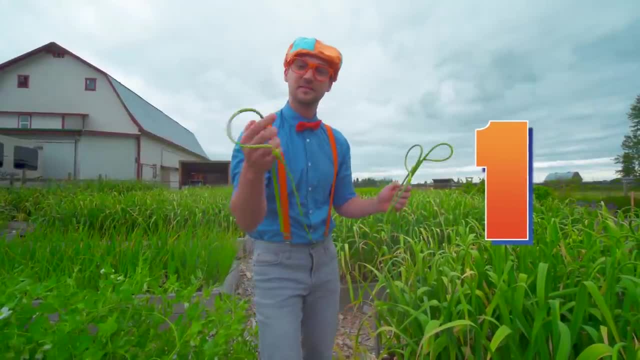 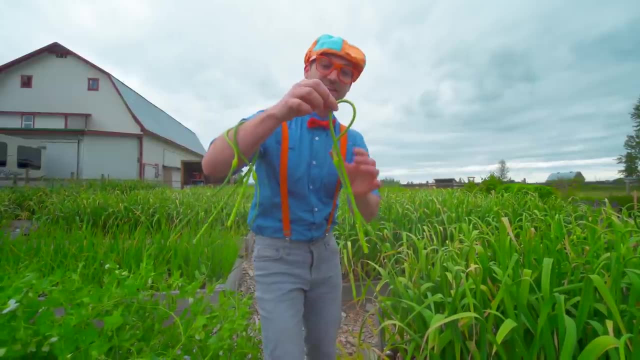 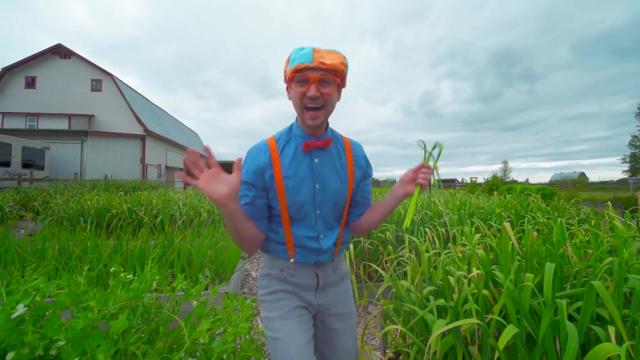 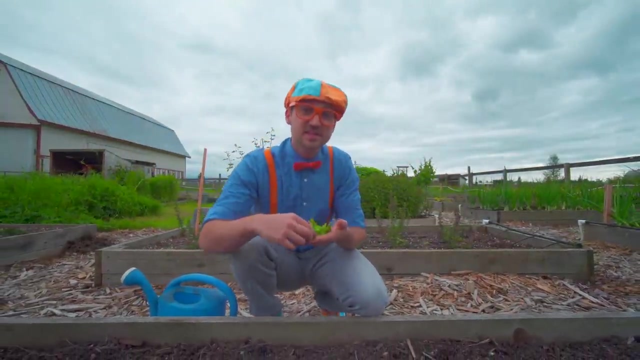 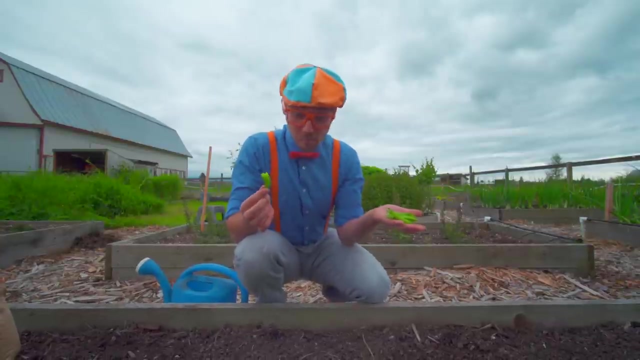 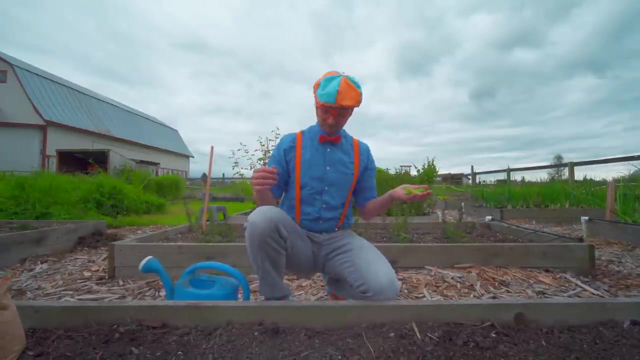 Let's count them All right. We have one, two and three, Wow, Three pieces of garlic top. Yum, Ooh. These are called snap peas, Mmm, And they're so yummy, Mmm. I think you and I should plant some snap peas. 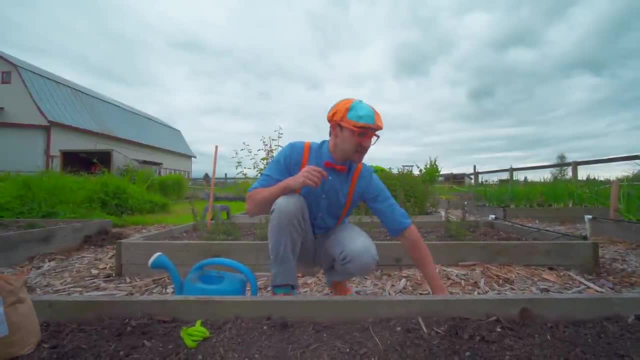 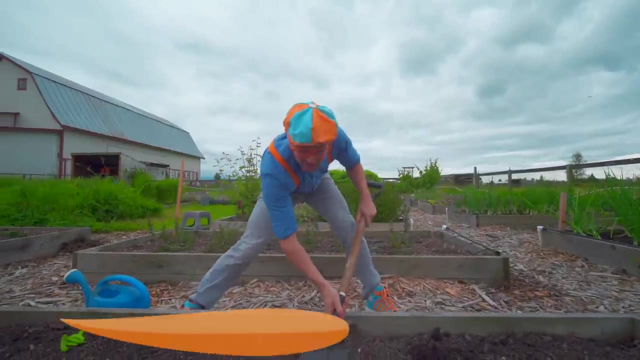 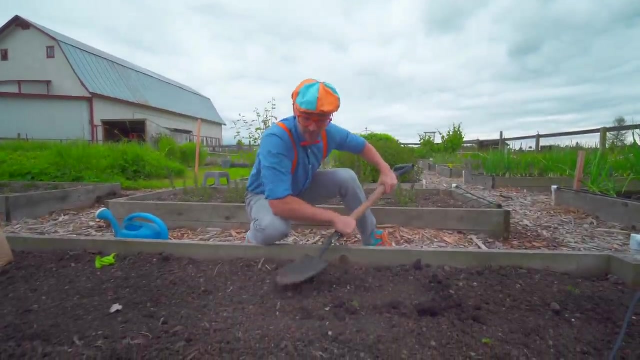 Okay. So to plant some plants, some plants, you need a shovel Where you dig a hole in a bed of soil, just like this, And put a seed right in the hole, Fill up the hole, Put some water on it. 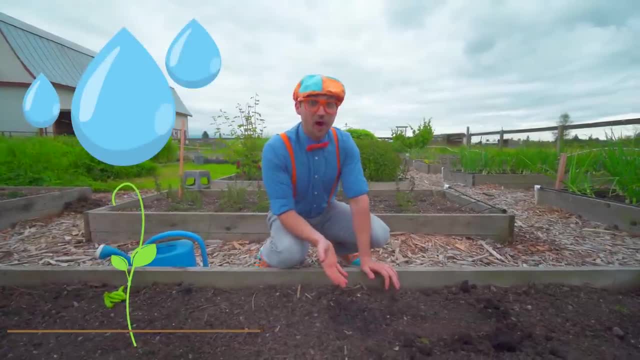 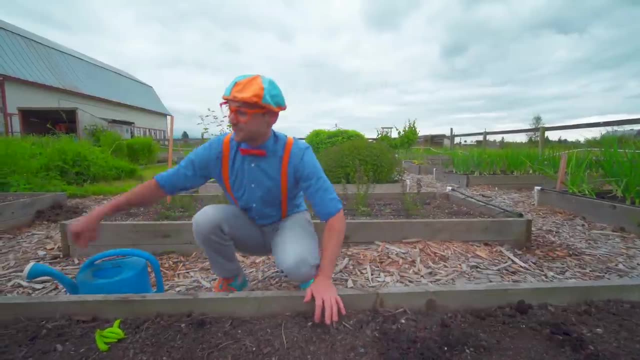 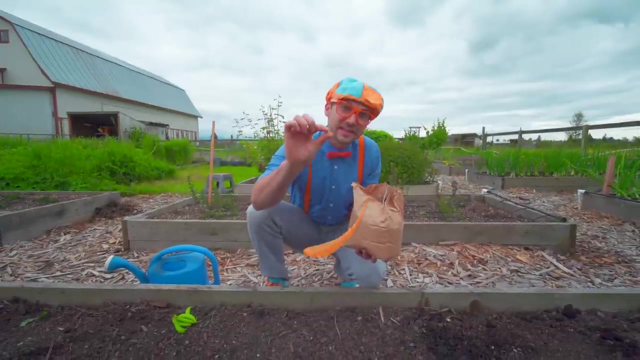 And then, after a lot of sun and some more water and a lot of love, it will grow into a tasty plant. All right, But for snap peas, all you have to do is put one of these plants in a box right on top of the soil. 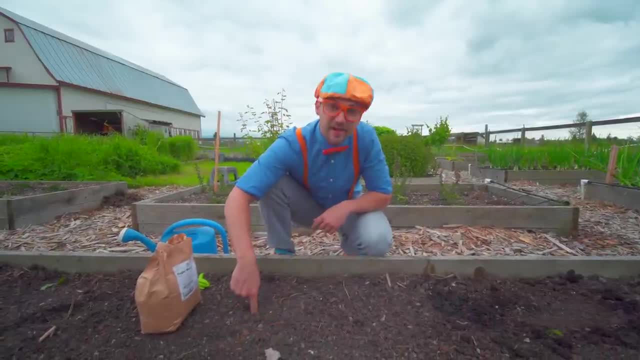 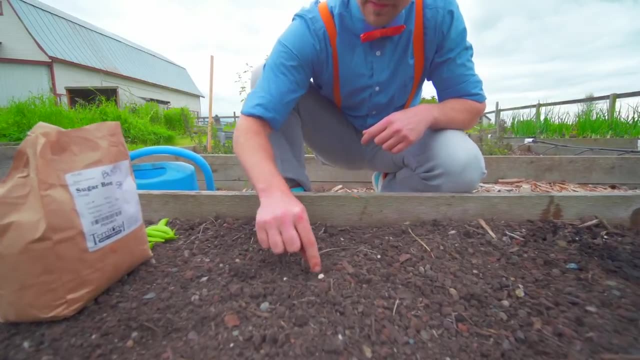 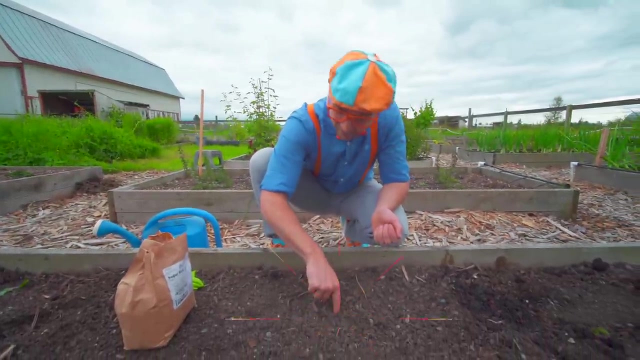 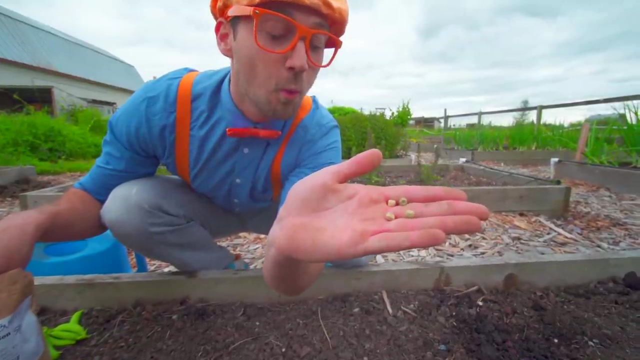 And push it down to right about there, Perfect. And then you take another one and push it down. Let's do a few more together. All right, This is really fun. Look at them, See. Let's count them. One, two, three, four. 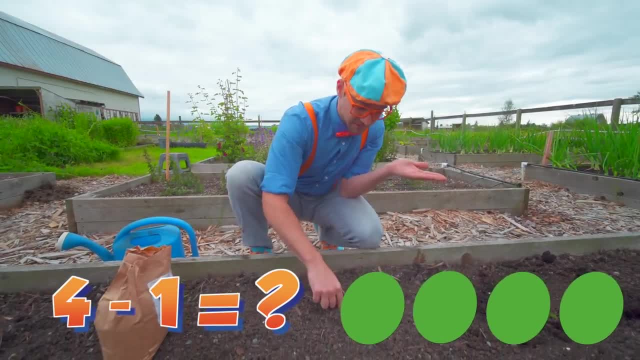 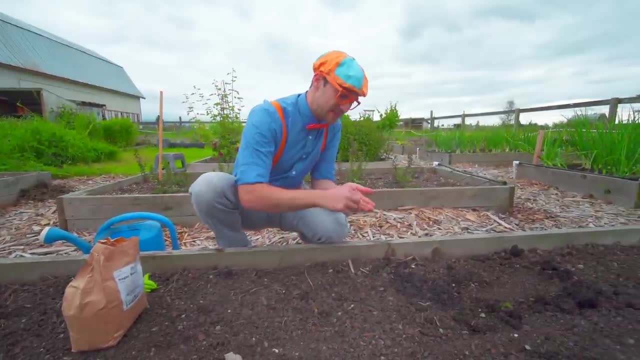 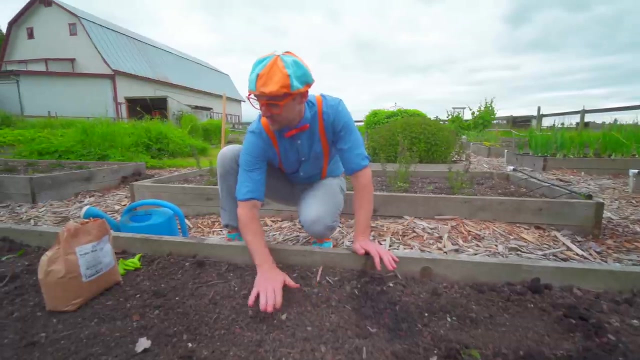 All right, Four minus one is three. Oh, All right, Let's put the rest of these down inside the soil. There we go, Okay, So we have a bunch of them right in a line right here, So let's move the rest of that. 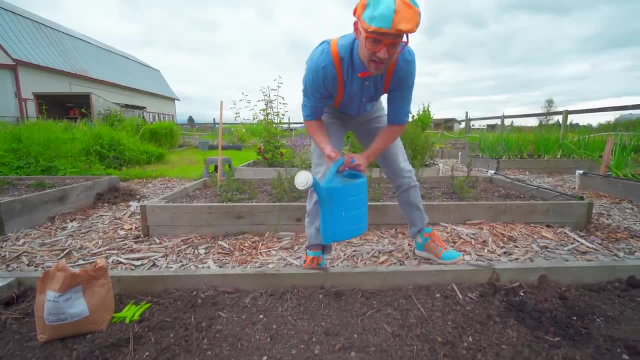 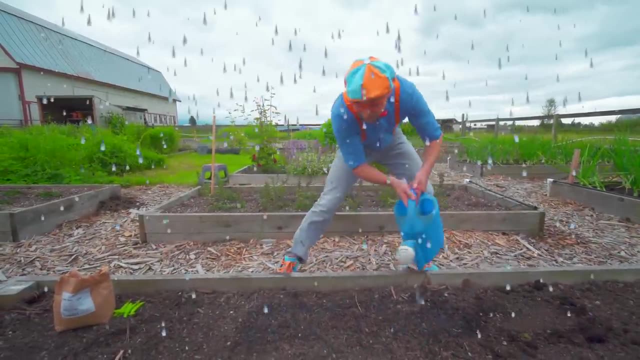 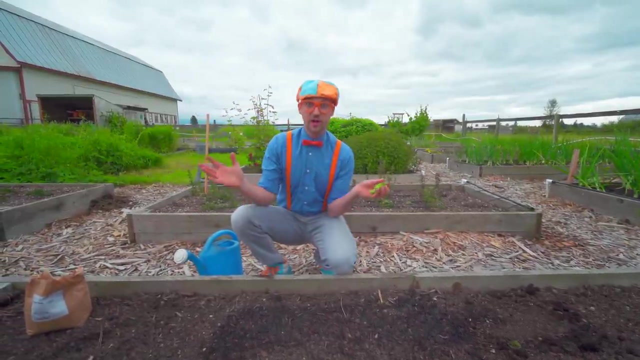 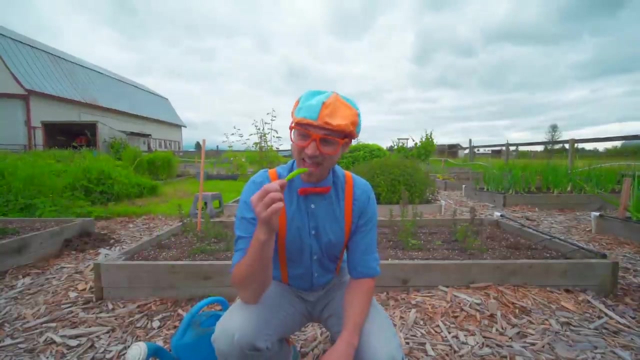 And those And let's take the water, And let's give them some water- Wow, All right. Then in a while these are going to grow into really big plants And then they'll grow these on them And then you can eat them like this. 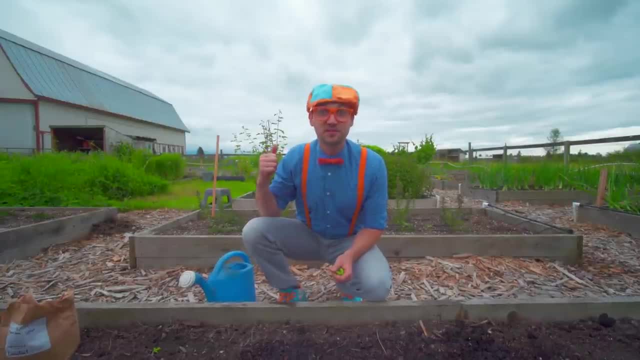 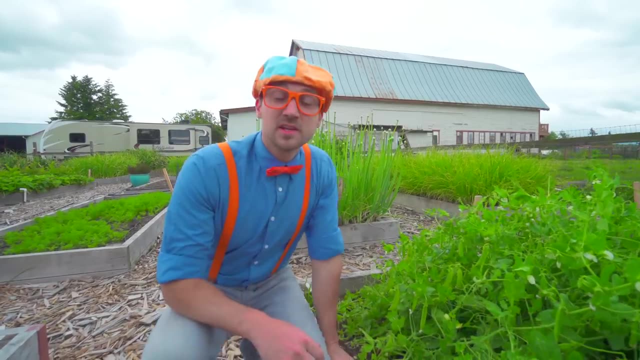 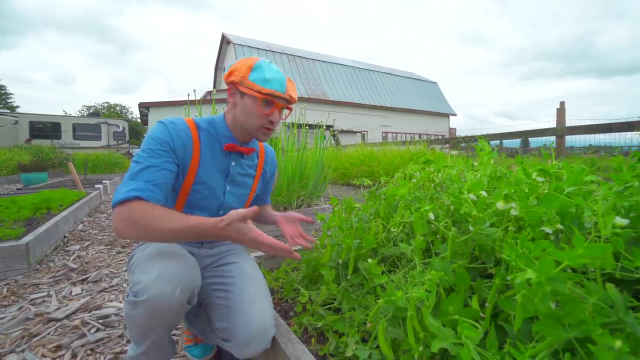 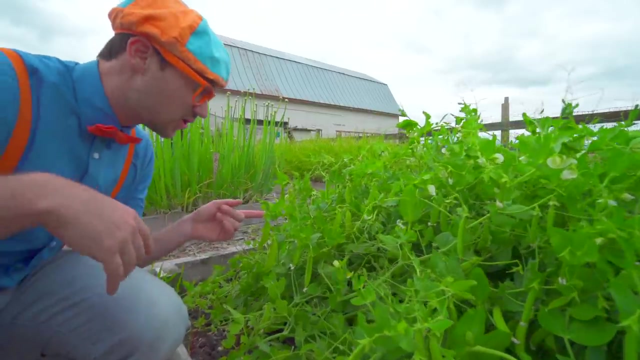 Wait a second. I think there's some big ones over there. Come on, All right. So those snap peas that we just planted in seed form after two months are going to grow to look like this. Look See, The plant has nodes. 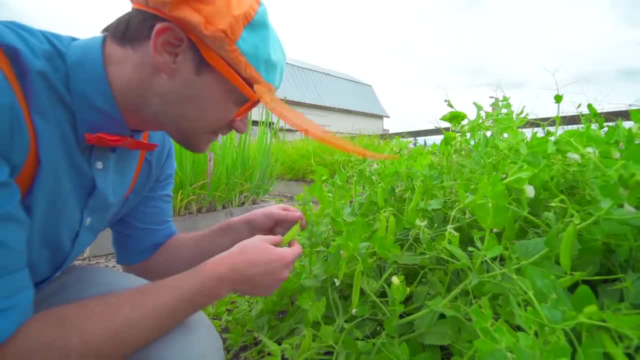 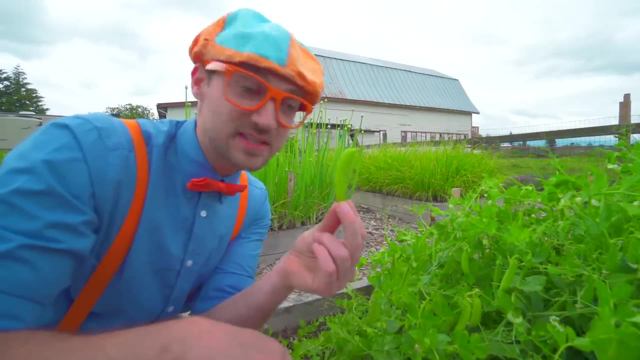 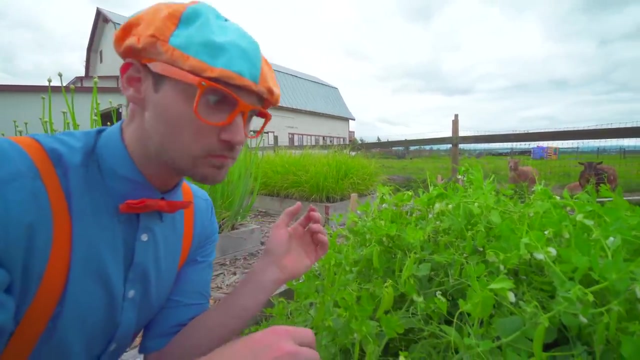 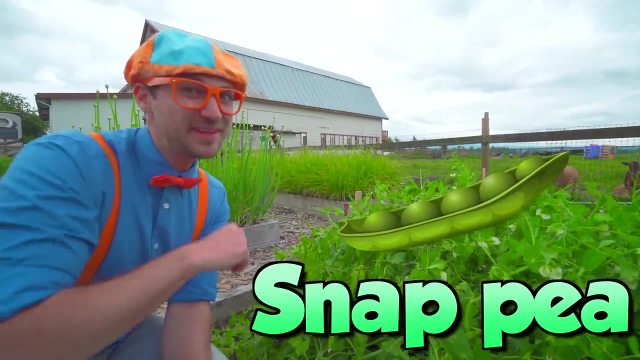 And then those nodes grow the snap peas off of them. Ooh, Pull it off And look, You have a lot of snap peas off this one plant. Hmm, Hmm, Hmm. Have you ever tried a snap pea? Maybe you should. 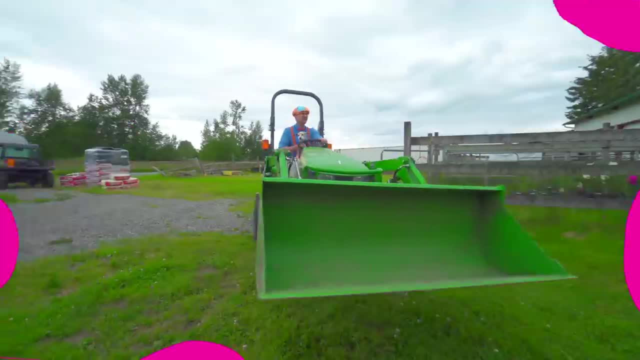 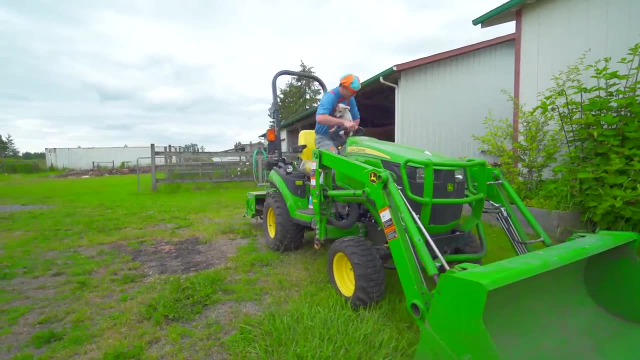 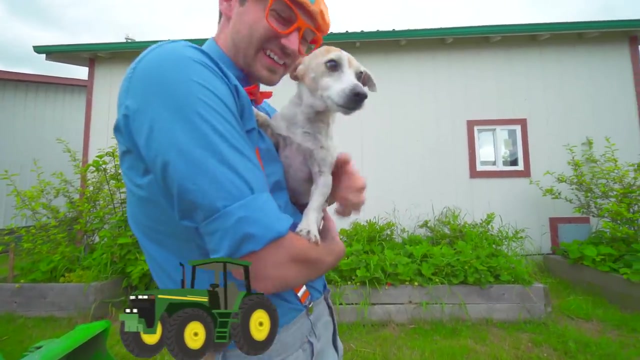 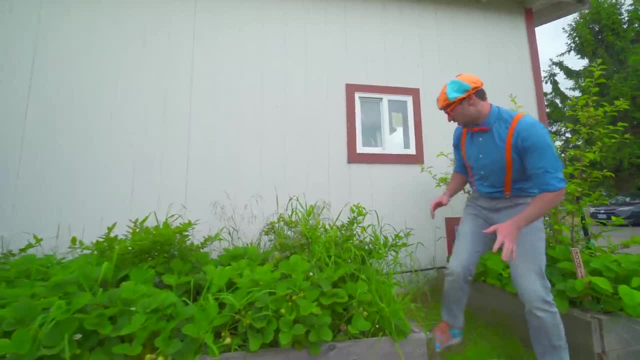 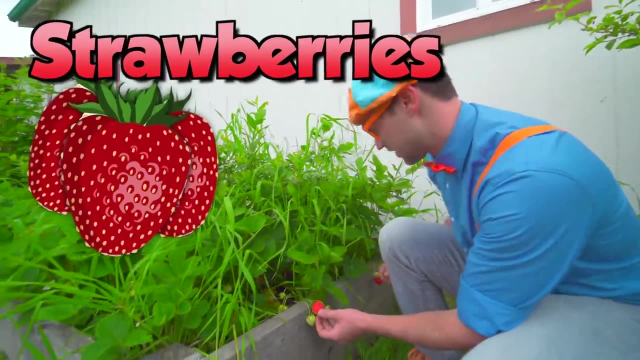 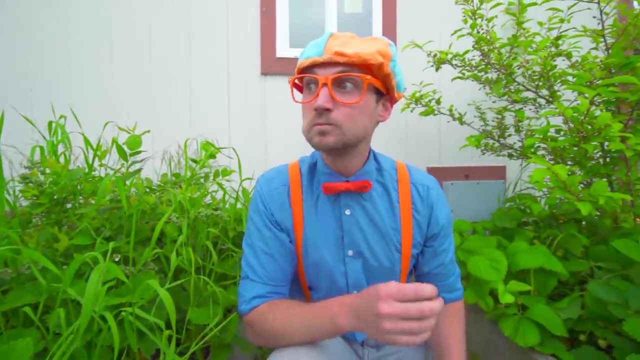 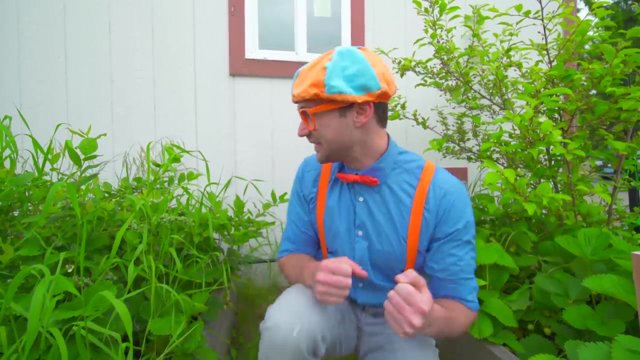 Come check this out. These are strawberry bushes. And look down here. These are strawberries, really red strawberries. Let me pull it off. Yum, Mm, mm. wow, that was tasty. Whoa, I love strawberry bushes. 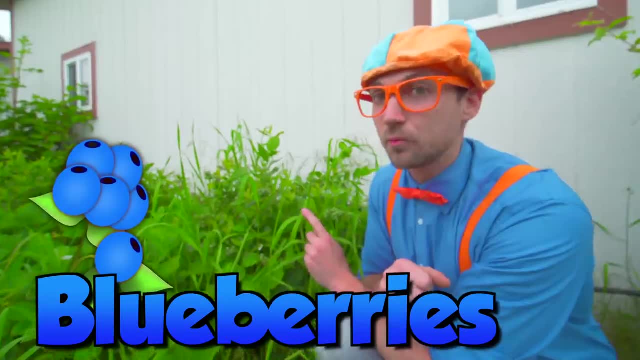 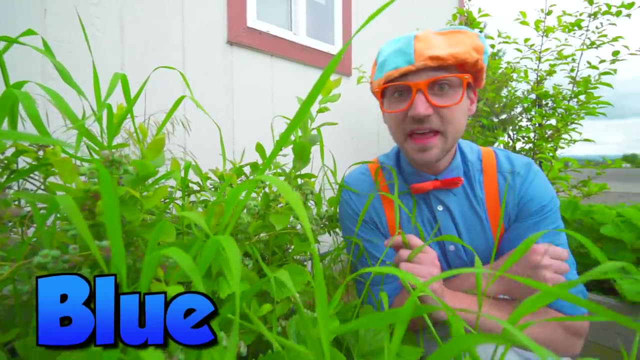 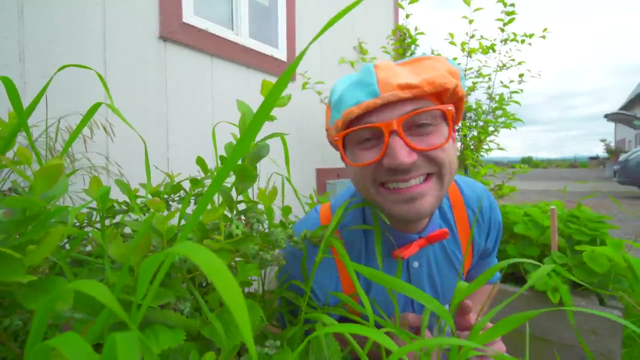 Ooh, and here's some blueberries, But they're not quite ripe yet. See these? Yeah, they'll be blue when they're nice and ripe, And then you can eat them. Ah, ah, Ooh, now we're in the chicken coop. 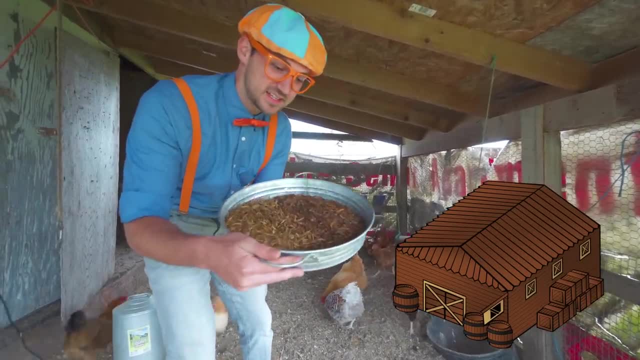 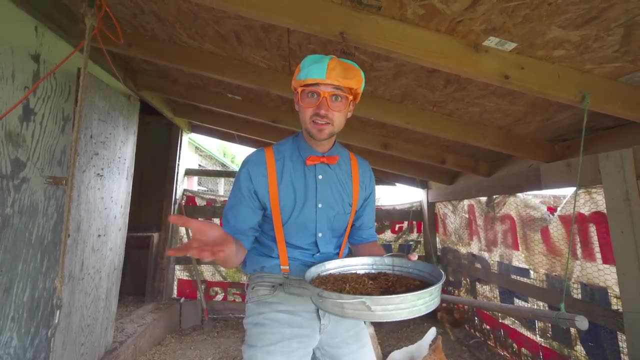 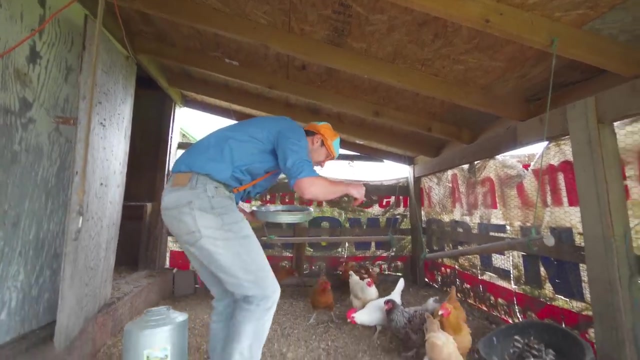 Hey, chickens, and look, These are some tasty treats for the chickens. They love to eat these tasty treats. so then they lay lots of eggs. I love eggs for breakfast, of course. All right, here you go, chickens, Whee, here you go. 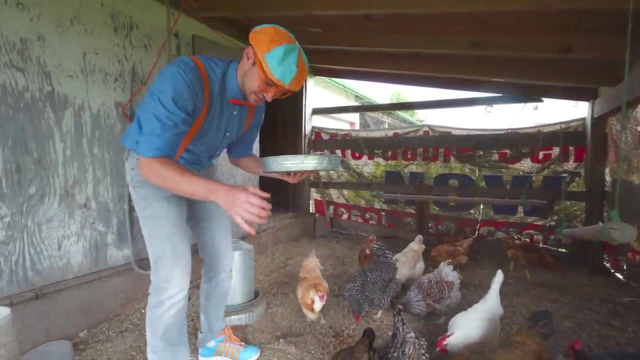 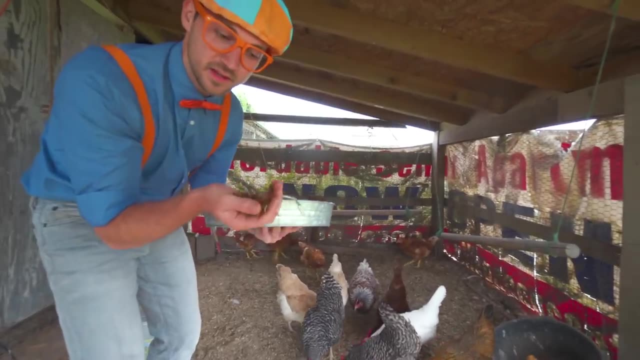 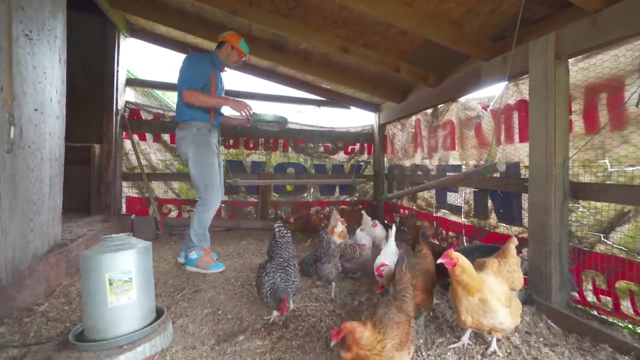 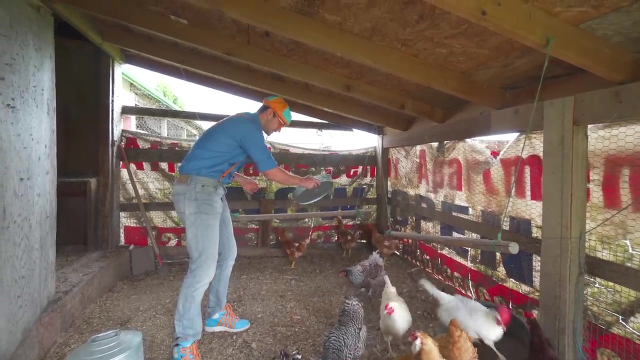 Ooh yum. They love these tasty treats, Just like how I love fruits and vegetables. these chickens love this stuff. I don't know what it is, though. Here you go, All right. all right, There you go, And from there you can spread the rust around. 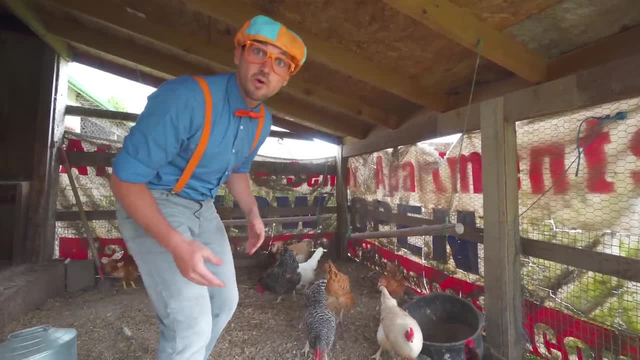 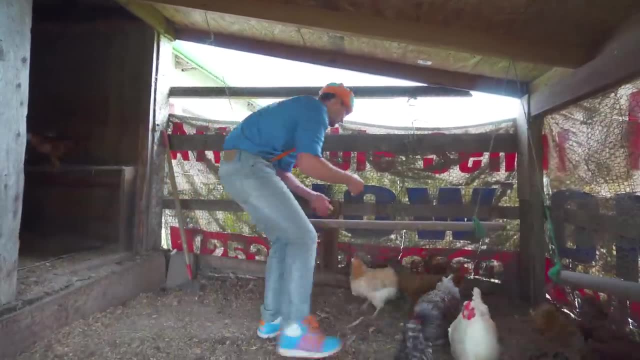 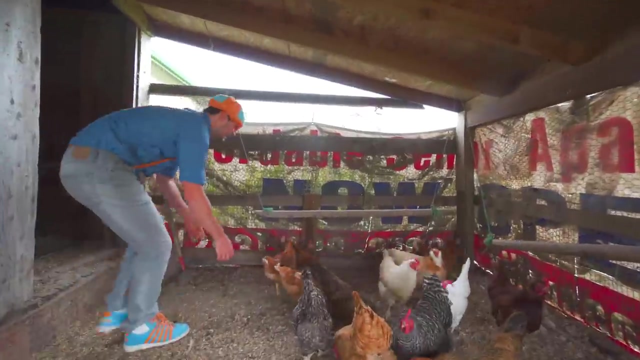 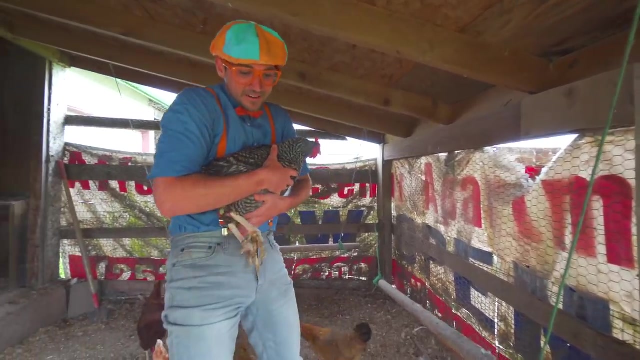 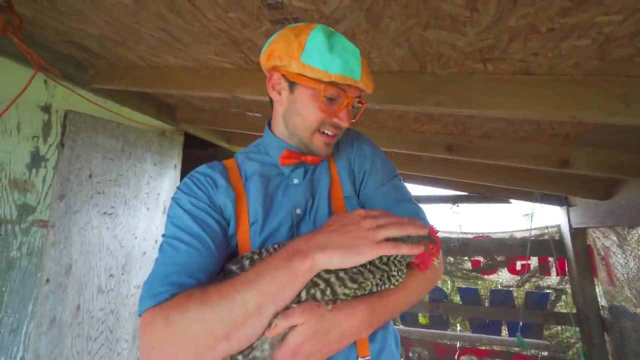 There you go, And now I'll pick one up so I can pet it. Oh look, I have a chicken and they love to be pet on their head. See, Hey chicken. Want to see the chicken? Oh, so cute. 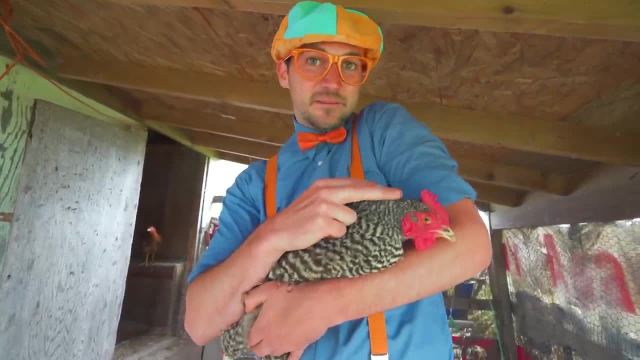 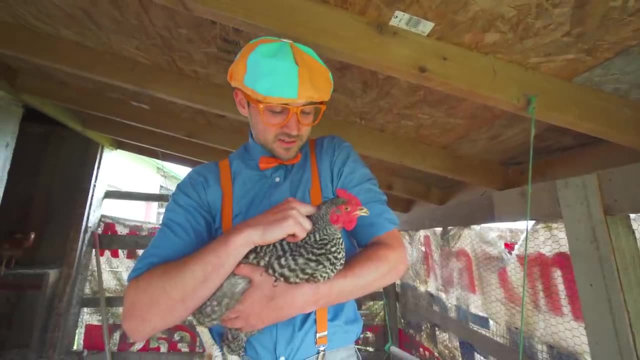 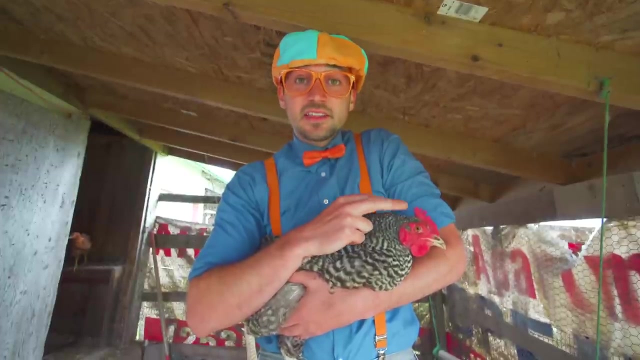 Their neck. Oh, so relaxed, So cute. Hey chicken chicken, Hey chicken chicken. See, Oh, it's okay, It's okay, girl See, the chickens live in this coop and they love to eat food, just like me and you. 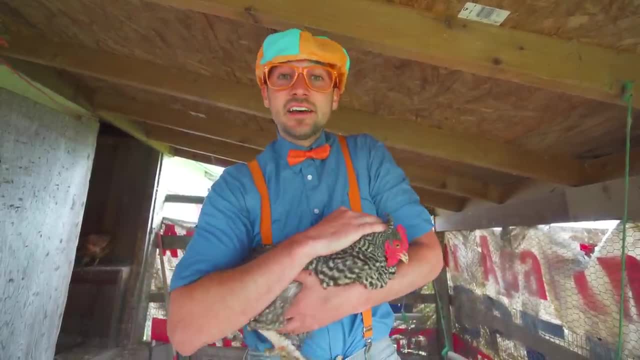 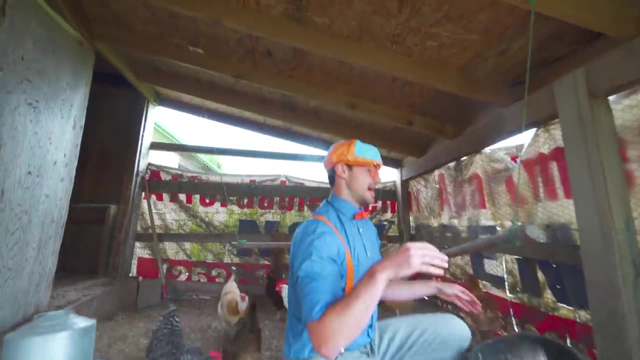 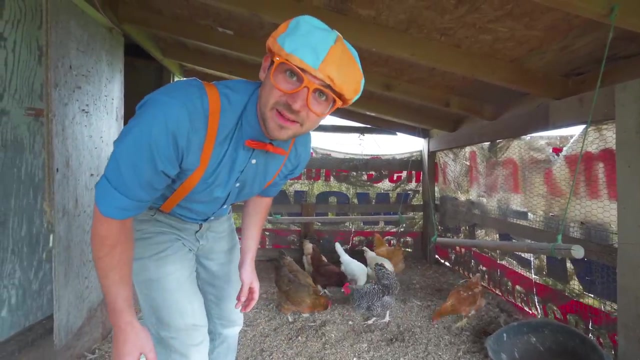 So then they can lay their eggs, so then you and I can eat them. They're so nice. All right, Here you go, Bye-bye, Have a good day. Time to pet another chicken. First we got to catch one. 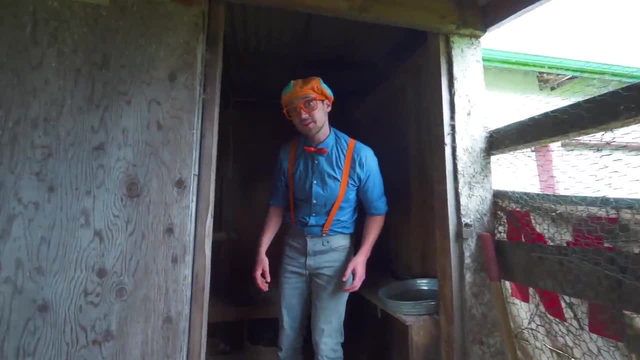 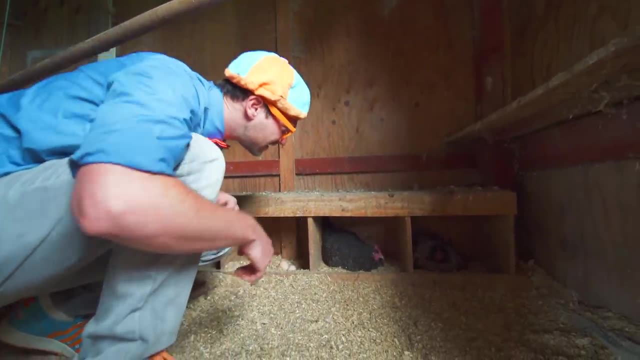 So now in this room, this is where the chickens lay their eggs- Come here, Whoa, See them down there. Yeah, they're laying eggs, And if you look right here, there's a couple eggs ready for us to grab. 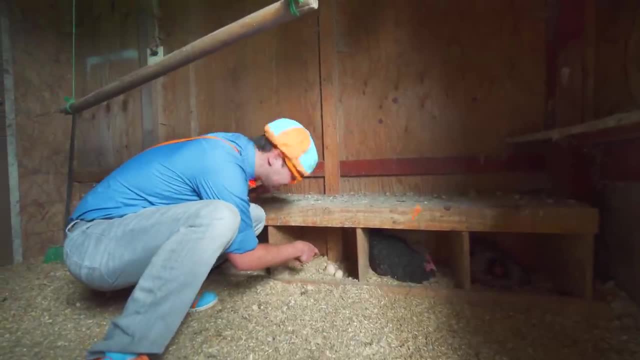 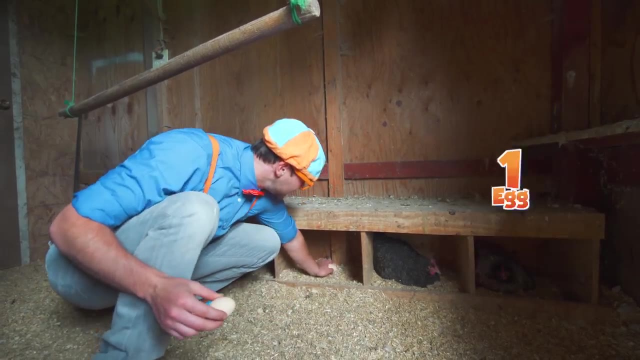 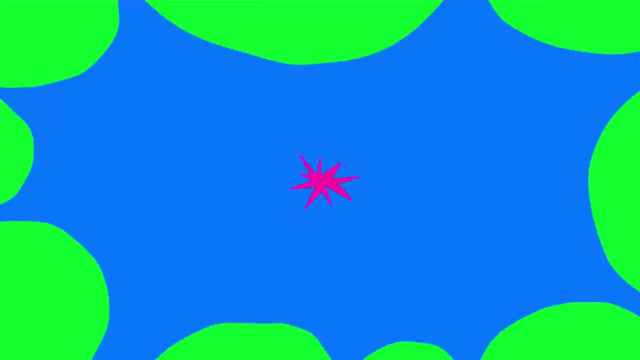 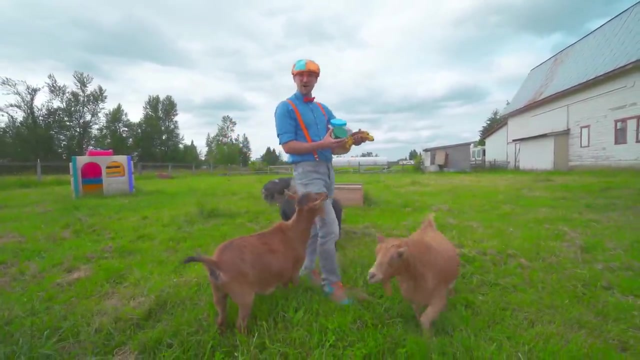 Look Right down there. One egg, Two eggs, Yum Whoa, One more. Oh look, look, look, Little chubby chubby. Hey Chubby, Hey Chubby, What's up? Hey pigs? 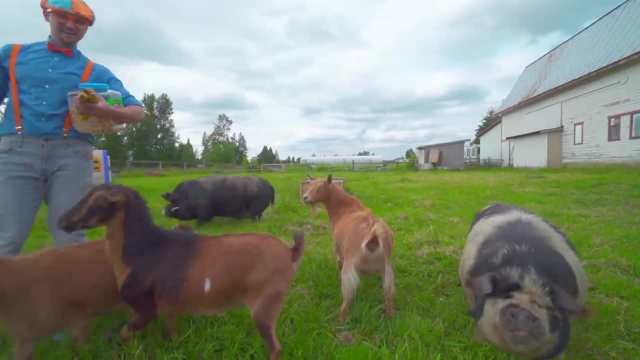 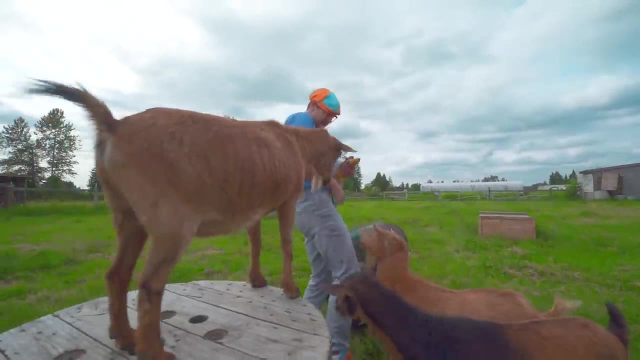 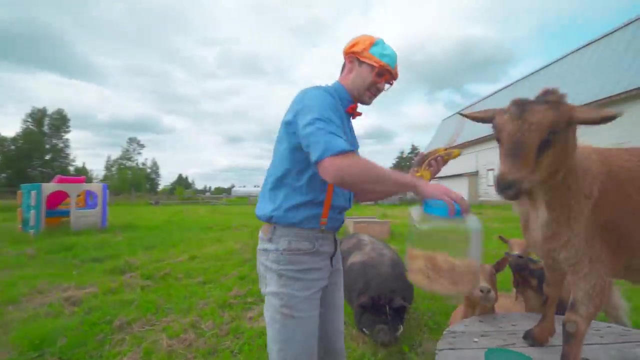 Another fun thing about this farm is they have farm pets too, just like these goats, Whoa, And there's some pigs back here. All right, Hey down whoopsies. okay, let's set some of this stuff down. i'm gonna set that down. all right, who wants some? 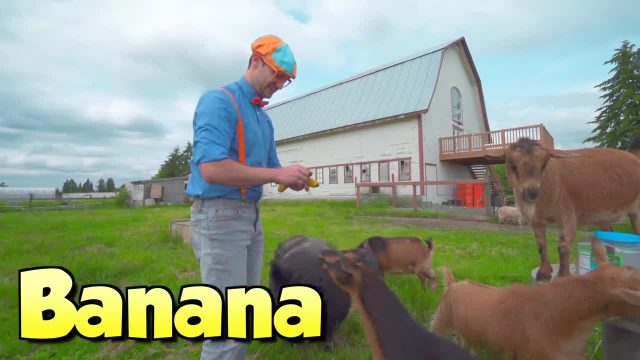 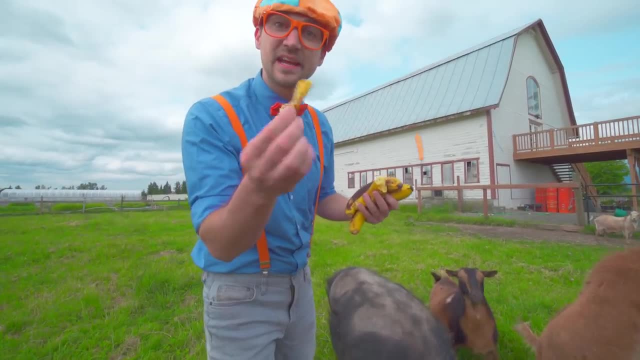 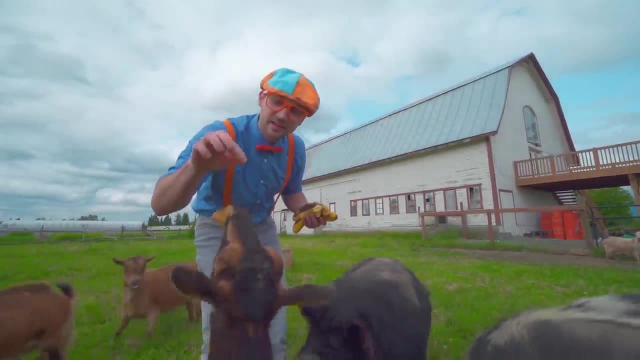 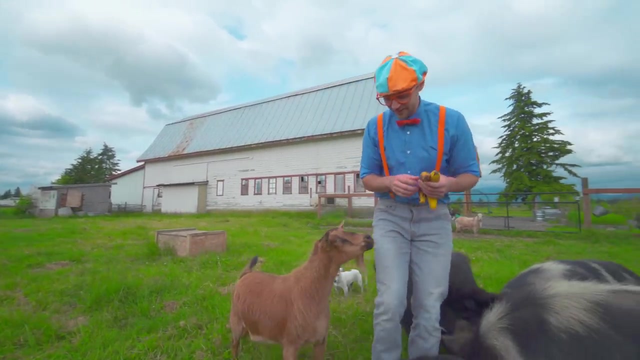 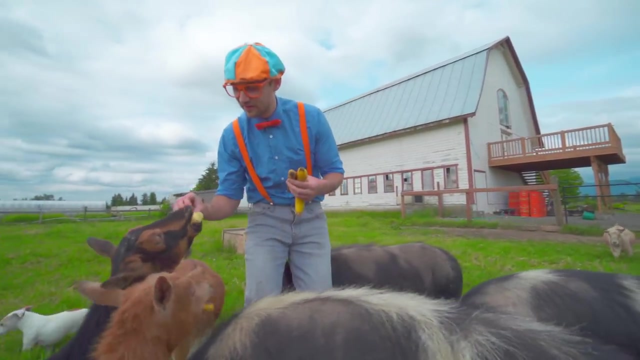 banana. oh yum, all right, would you like some banana? oh, there you go. oh, you know the banana peel part that you and i don't like. they love it. check it out. you want it. yum, would you like some banana? yum, enjoy, would you like some banana? okay, there you go. okay, hey, this one hasn't got any, hey, would you? 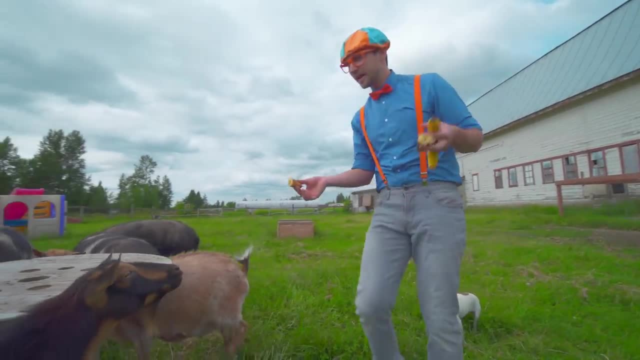 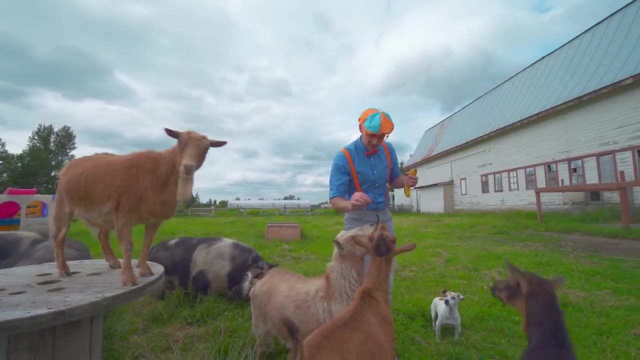 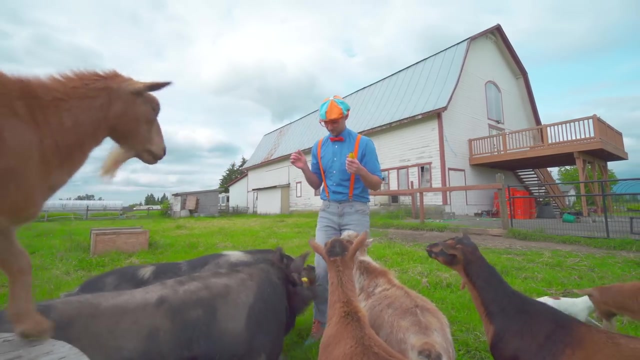 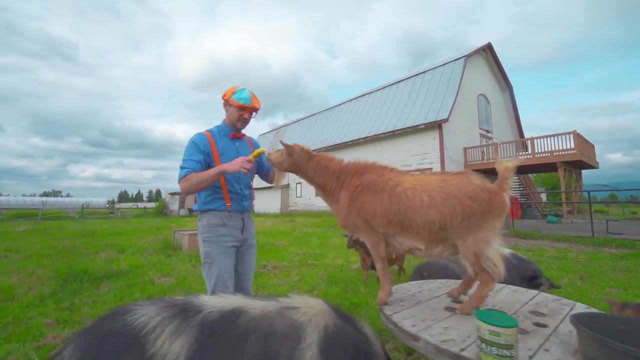 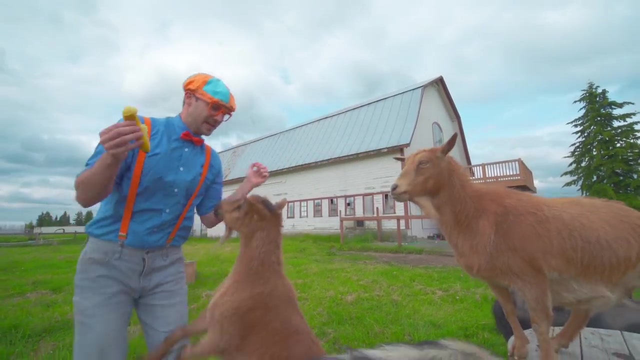 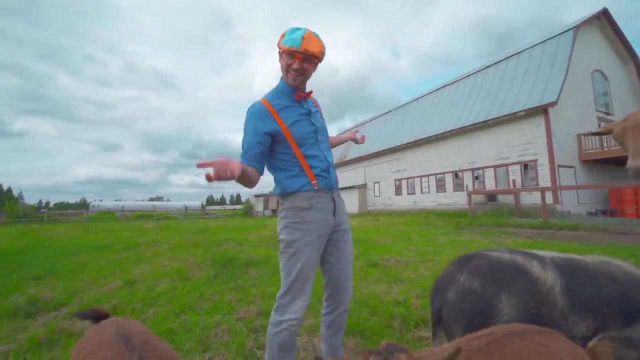 like a treat? hey, oh hey, would you like a treat? oh, hey, down, good, down there you go. hey pig, hey pig, there you go. oh, all right, would you like some banana? there you go? all right, there's some peel for you. eight down, put it down. all right, here you go, you two can share. sharing's really good. oh, here's some more treats over here. 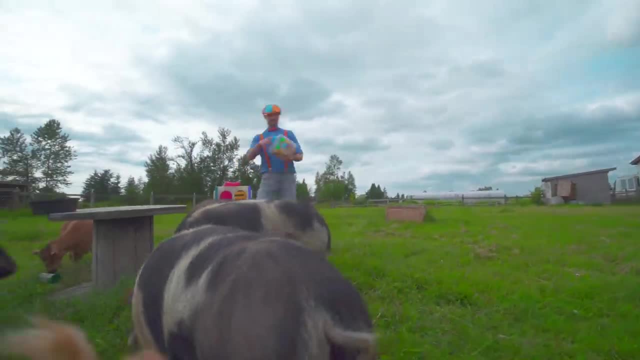 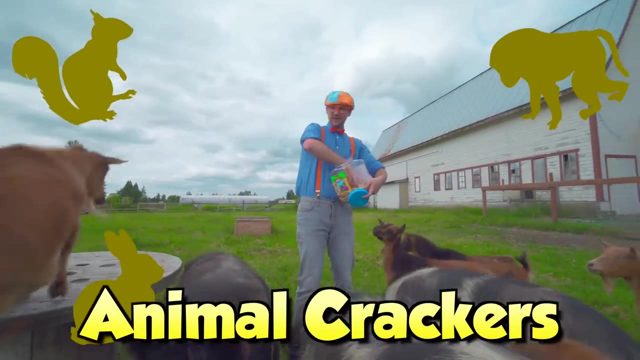 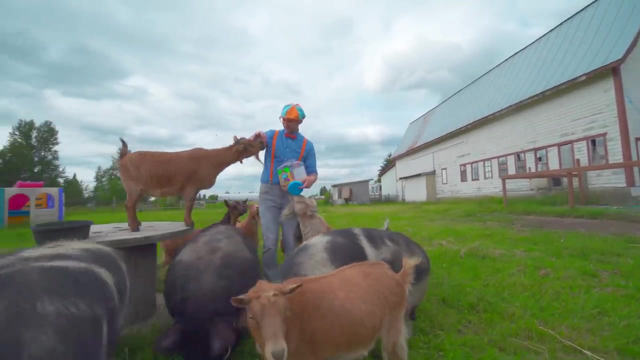 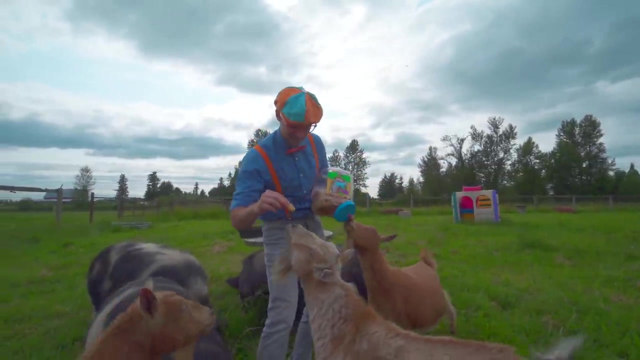 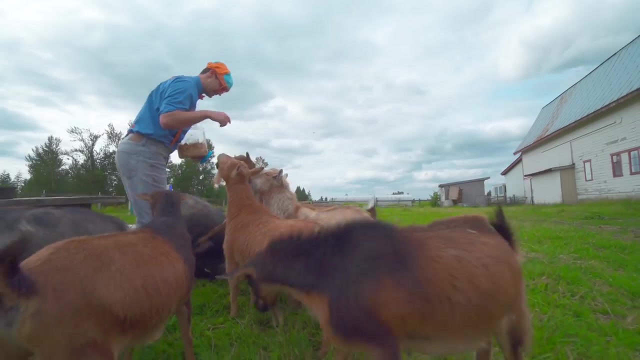 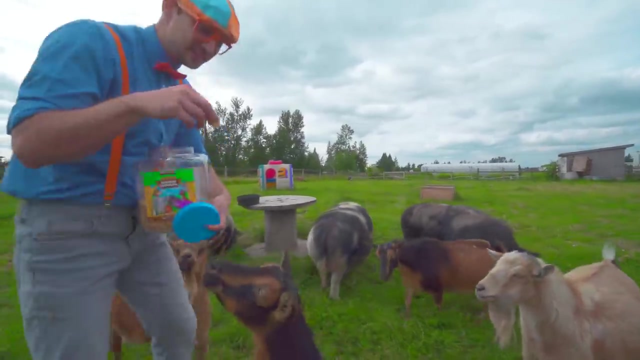 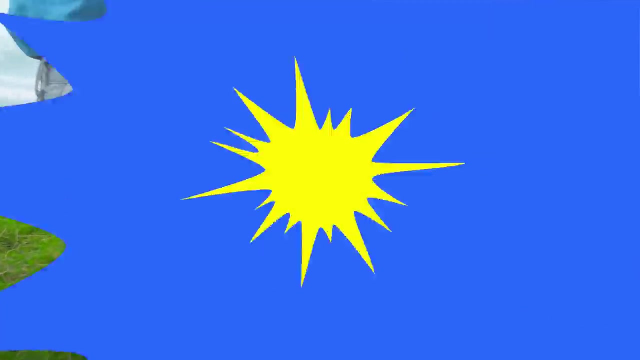 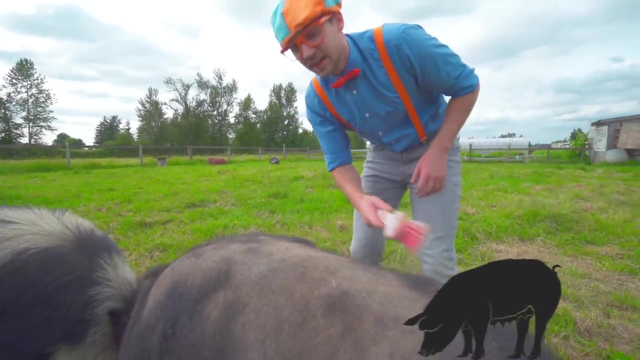 oh look, animal crackers. all right, who wants some crackers? there you go, here you go here. see, it's an animal, but it's a cracker. here you go. hey down, put it down. you see what i'm doing. i'm using this brush to give him a nice back scratch. 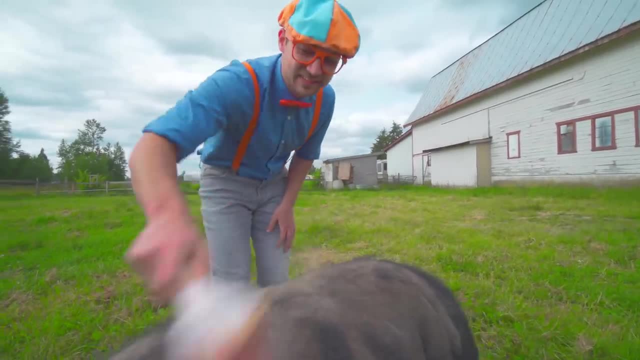 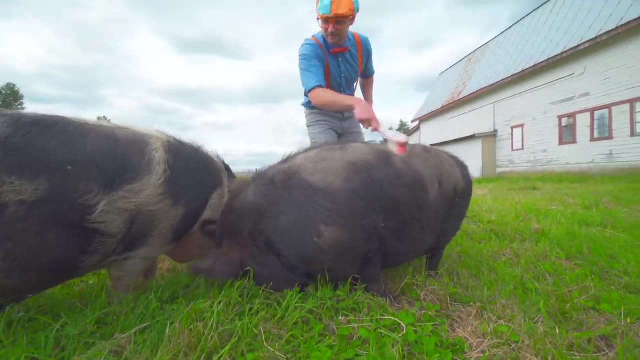 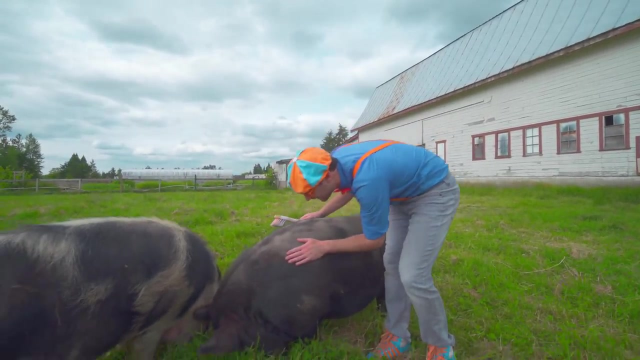 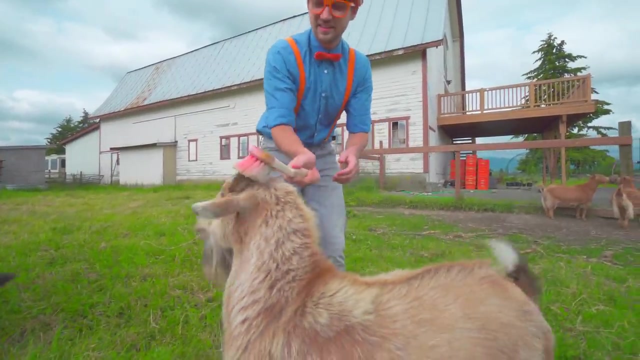 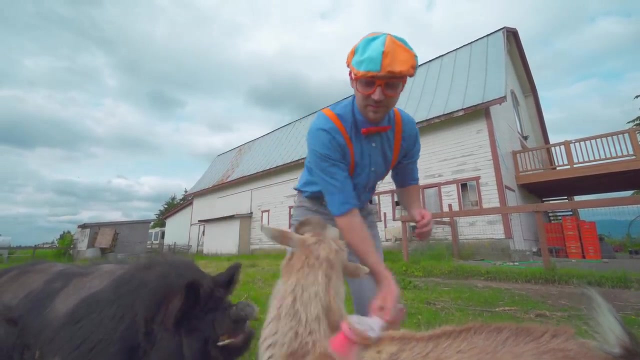 there you go. hey, ooh, does that feel good? yeah, have you ever gotten a back massage or a back scratch? yeah, this probably feels just like that right pig whoa the skin. hey, would you like to get brushed? yeah, there you go. there you go. oh, yeah, does that feel good? it's kind of like a bath, but without water, and it doesn't clean you. 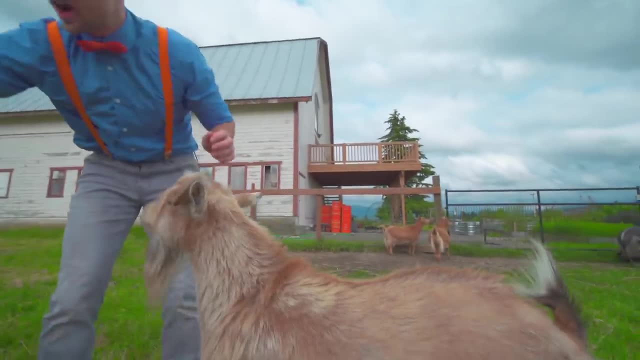 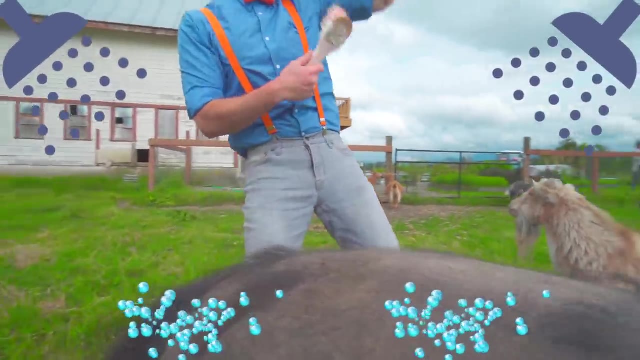 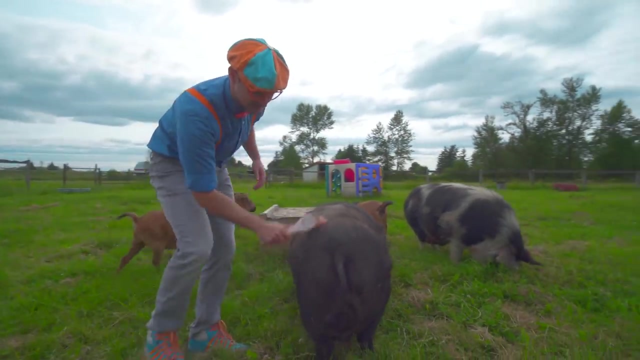 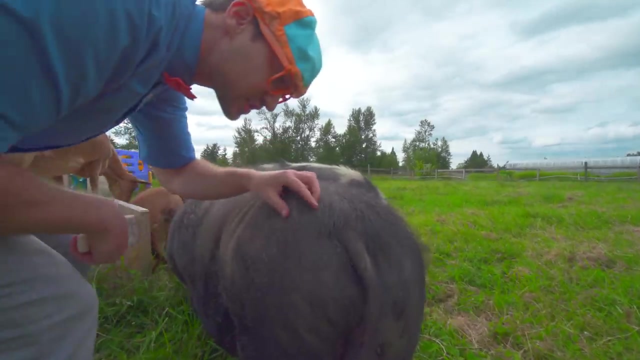 it just feels really good. i like taking baths and showers nice and clean, rubbing a brush on my skin. okay, here you go, let's get you right there. come check out this pig's hair. whoa, it's really coarse and really thick. wow, it's really thick. 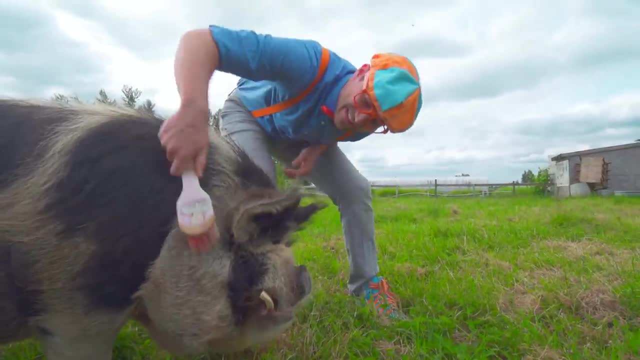 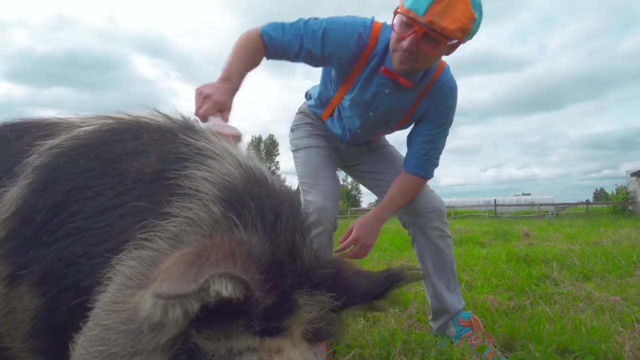 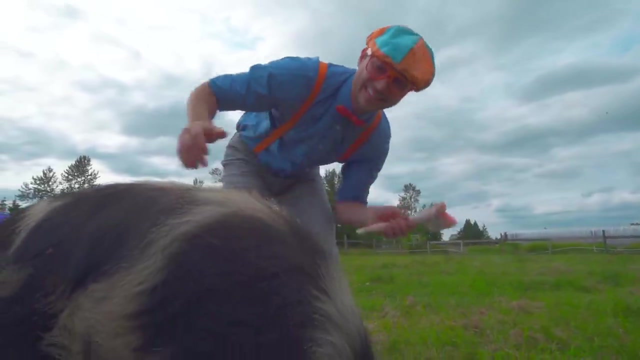 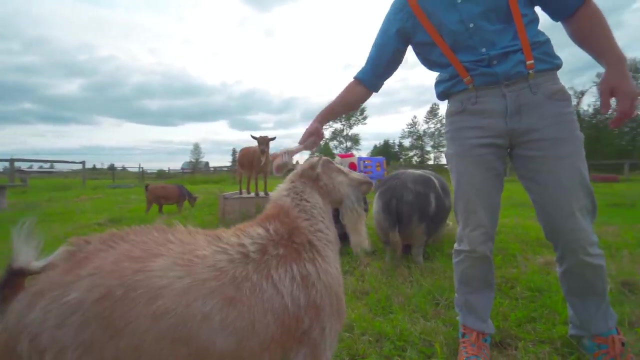 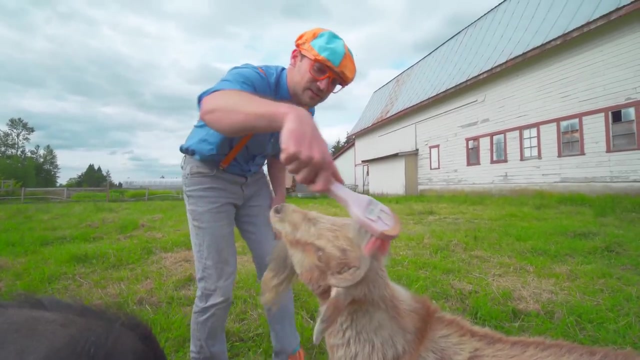 hey pig, there you go. oh, yeah, does that feel good? oh, i bet, there you go. yeah, see, i'm brushing this pig. this pig is really big. whoa, can i give you a hug? does that feel good? yeah, that feels real good. you like your horns brushed? huh, yeah, there you go. 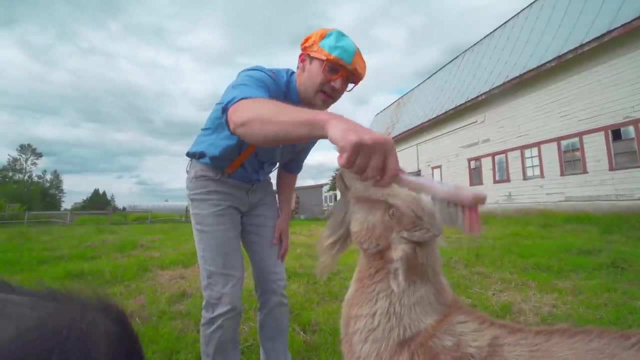 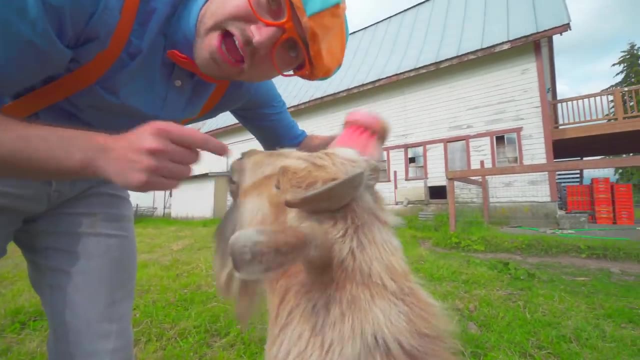 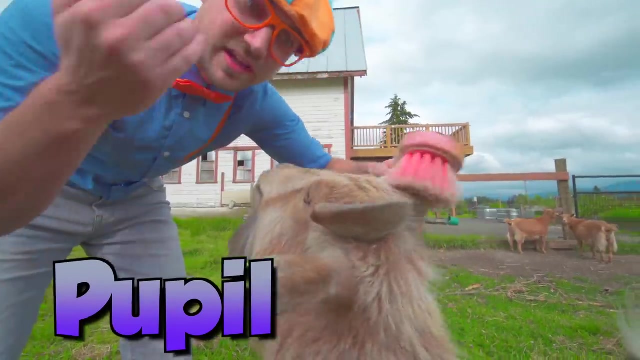 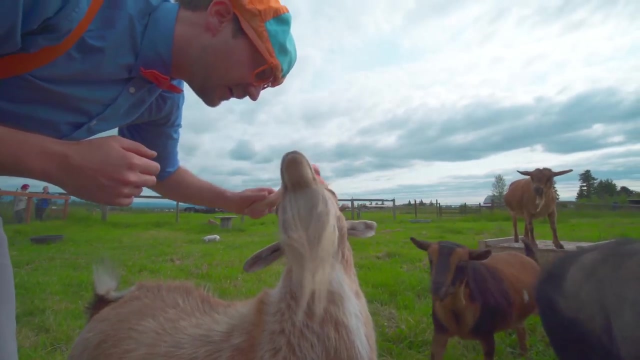 you're a nice guy, whoa, and do you see his eyes? look, look at his eyes. come here. do you see the black pupil? yeah, that black part is called the pupil, and it's sideways. so then, from there, the goat can see all around itself. wow, there you go, buddy. all right, have a good day, bye-bye. 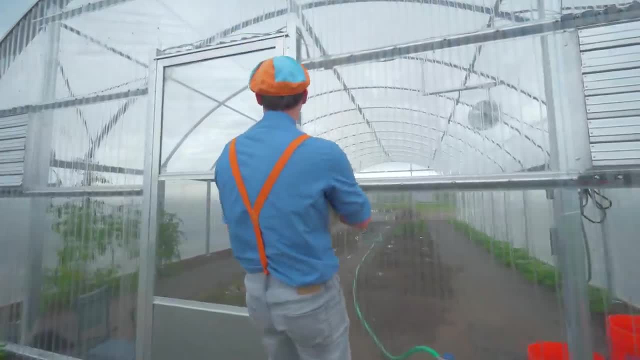 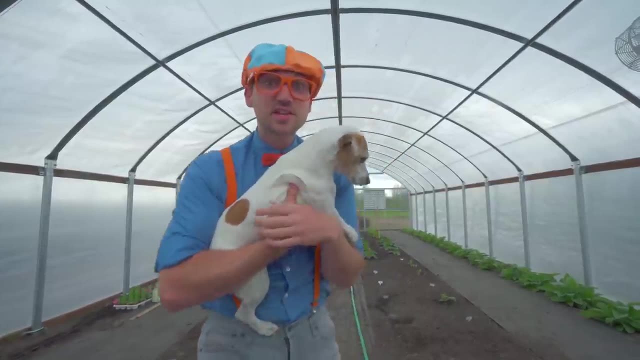 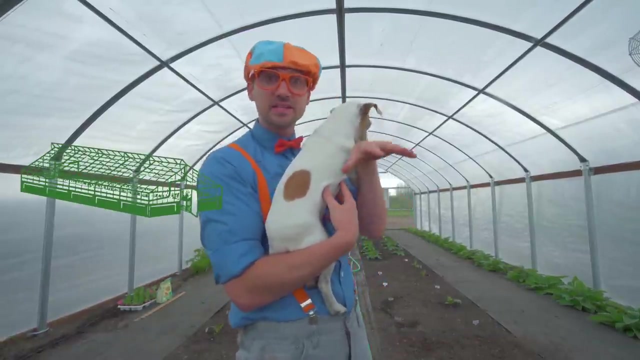 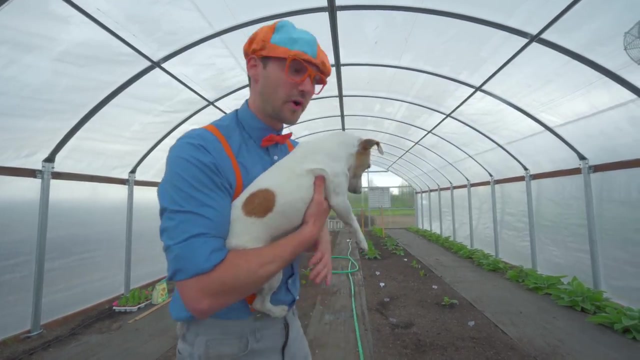 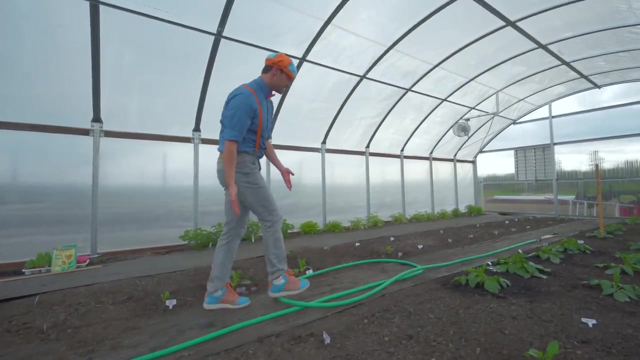 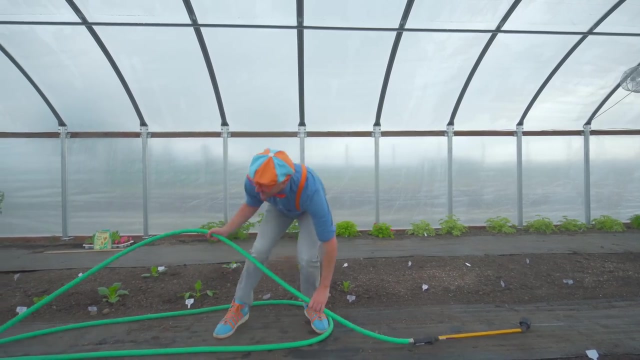 bye-bye. oh, what's in here? wow, this is a growing room. growing rooms are kind of like greenhouses: they keep a little bit more heat inside than outside. right, sheila? all right, let's go explore. oh, look at what it is. it's a green hose. whoa, oh, hey, look at what's on the end of the hose. 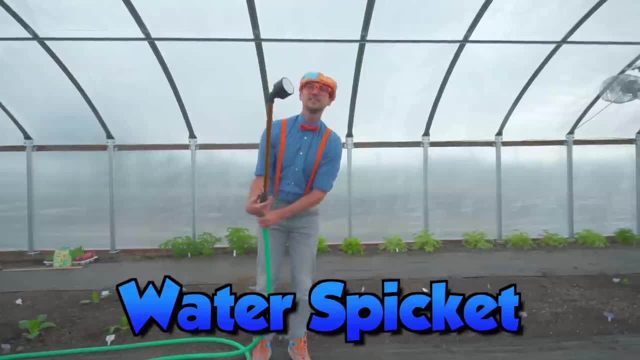 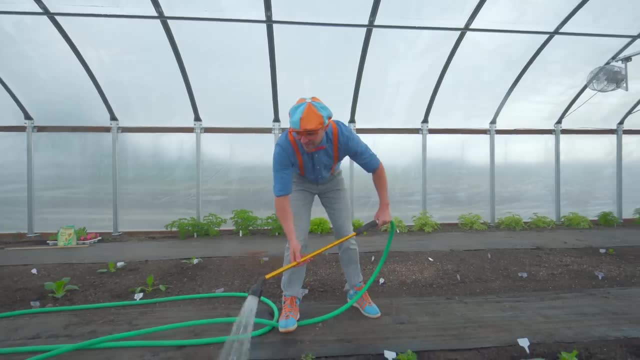 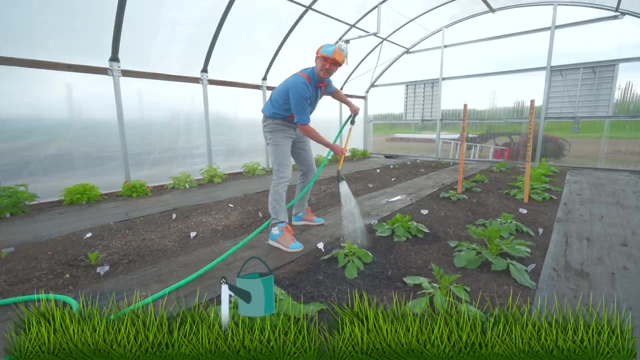 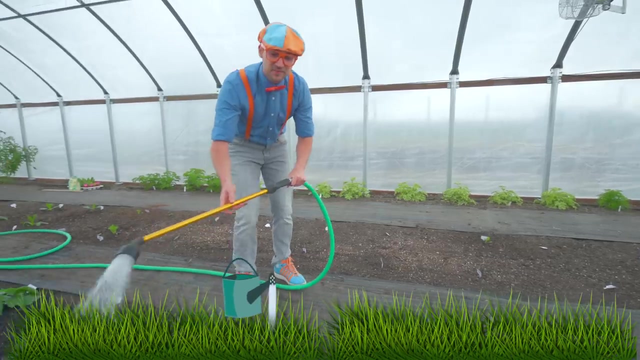 oh, it's a watering spigot. what does it do? whoa? it sprays water. let's water the plants there you go, there you go. yeah, plants love to drink water, just like you and i do. all right, wow, this is so much fun growing plants. 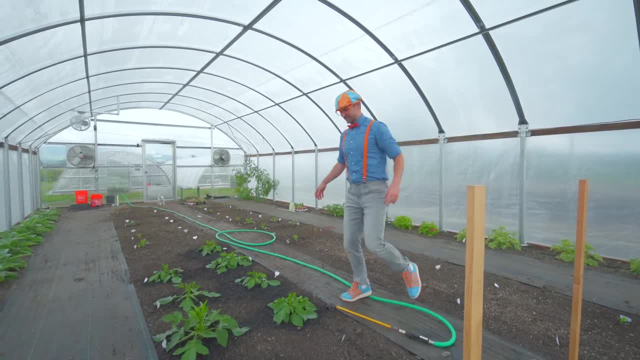 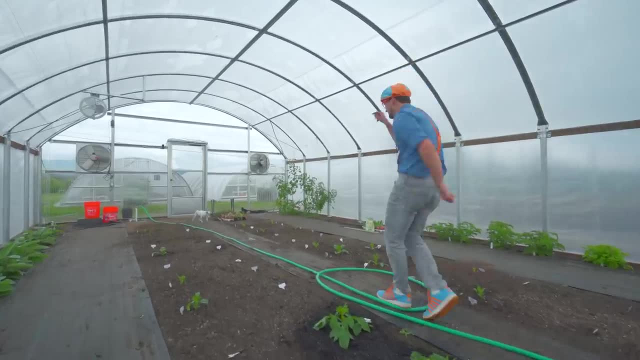 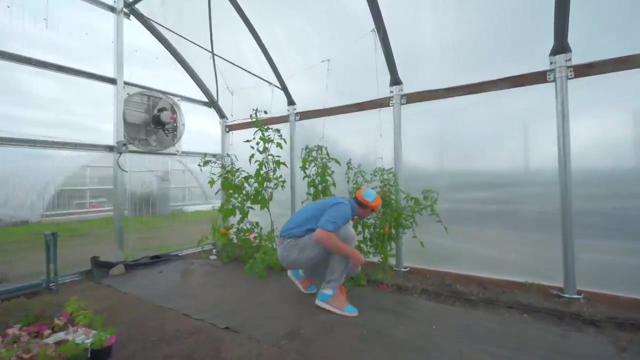 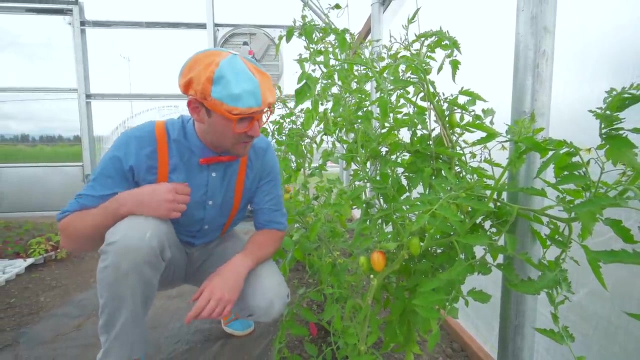 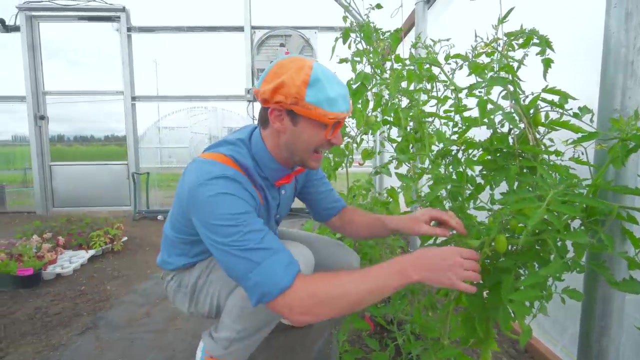 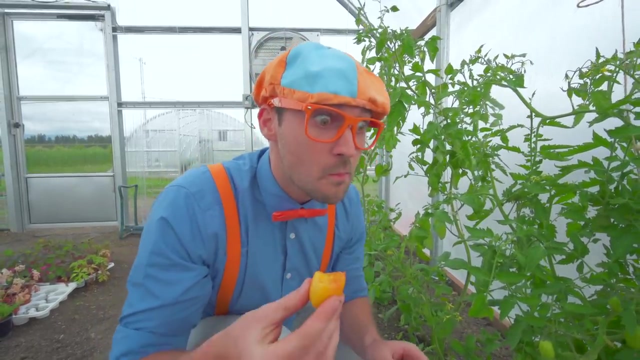 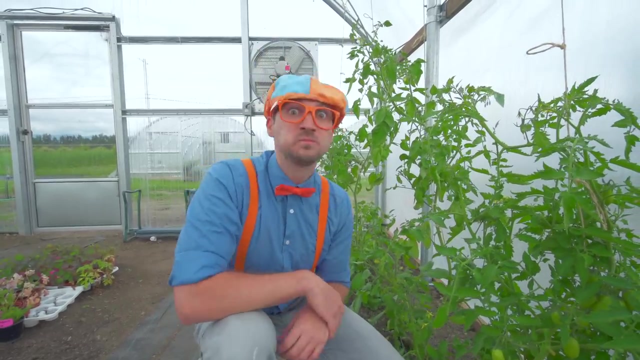 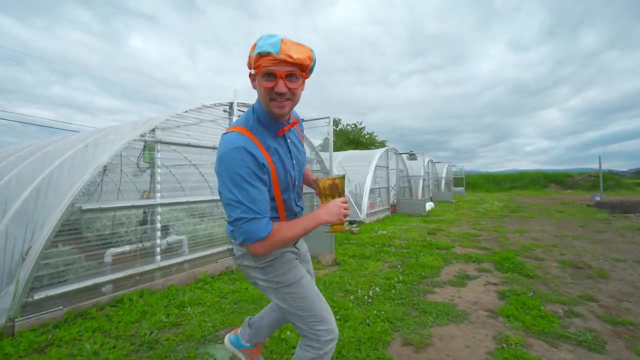 because i love to eat the food afterwards. speaking of food, look way down there, oh look, oh, it's a plum tomato. oh, it looks so tasty. shall we eat it? wow, yum, hmm, yum, hmm, oh. another fun thing to do at laughing goat flower farm is to make a bouquet. come on, 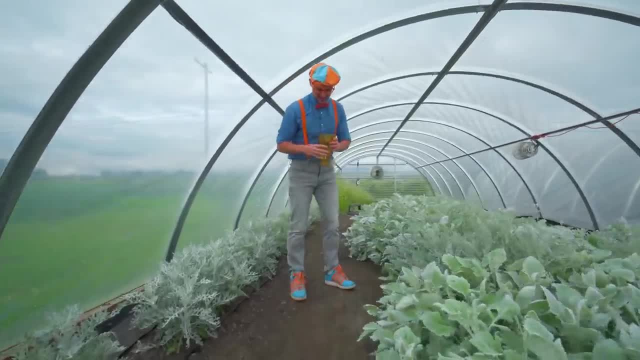 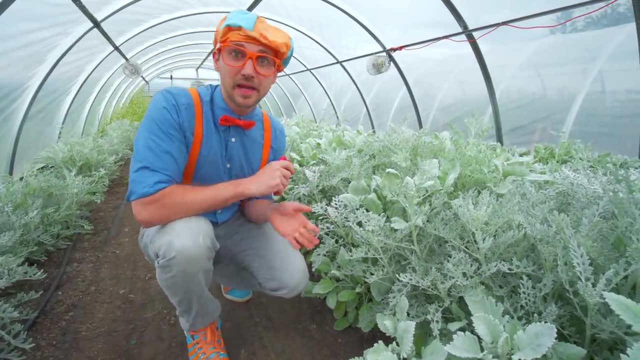 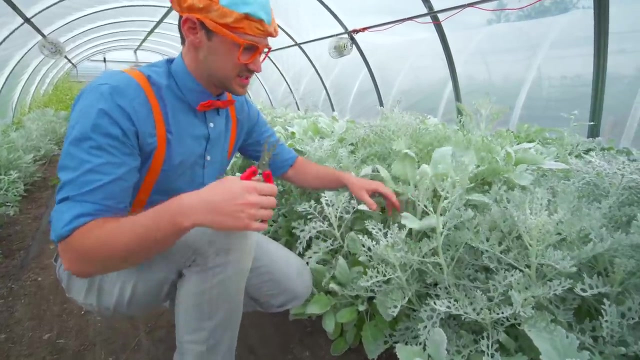 whoa, look in here, some more plants. all right, so these plants you don't eat. yeah, these plants you make a beautiful, beautiful bouquet with. all right, here we go, let's take our snips. all right, where to go. How was your day? Got some nice flowers? here we go. some nice flowers, here we go, let's take our snips. all right, where to go? How about a plastic flower? flower. 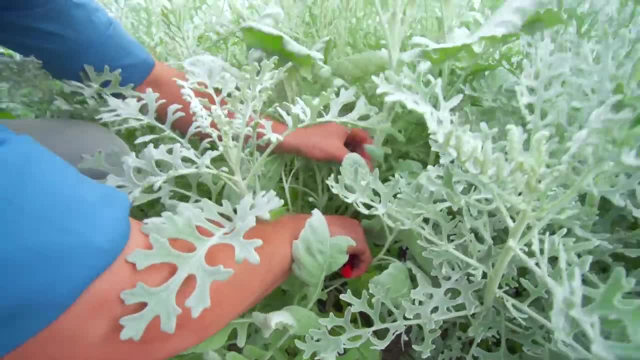 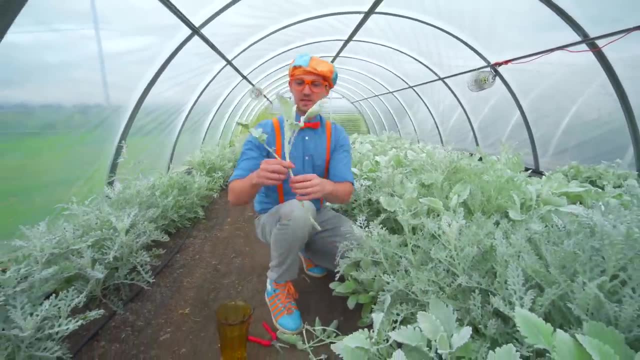 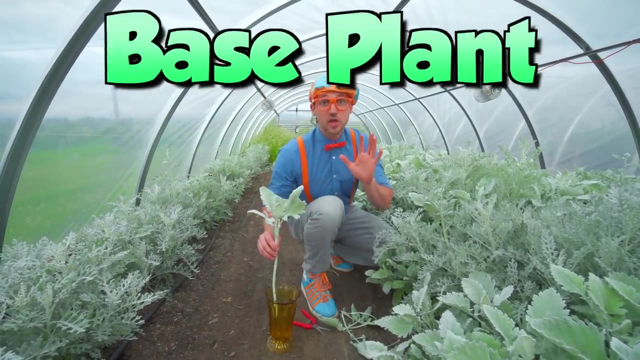 How about, right there, All right, Okay, Oh, that's real pretty. So how you make a bouquet is you start with a base flower like this. Well, actually, you start with a base plant and then you add the beautiful colorful flowers. 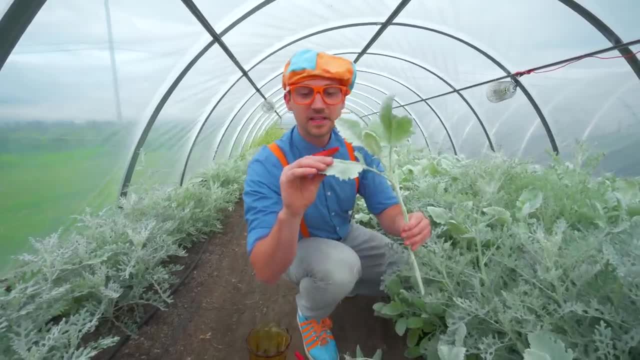 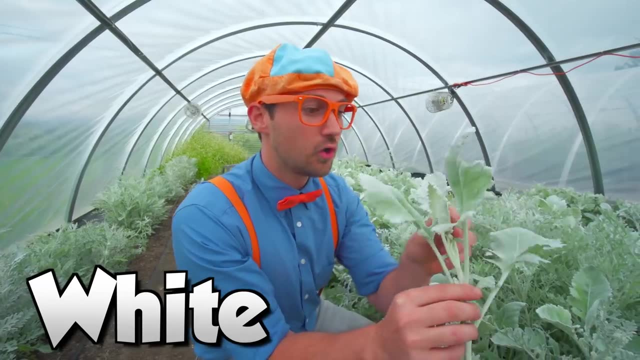 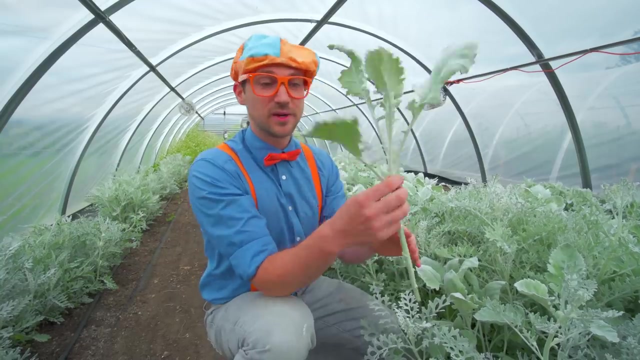 But this plant right here? yeah, it's fuzzy And it kind of looks like the color white. Yeah, Normally plants are the color green. Well, sometimes It really depends on the plant, But this one is pretty white looking. 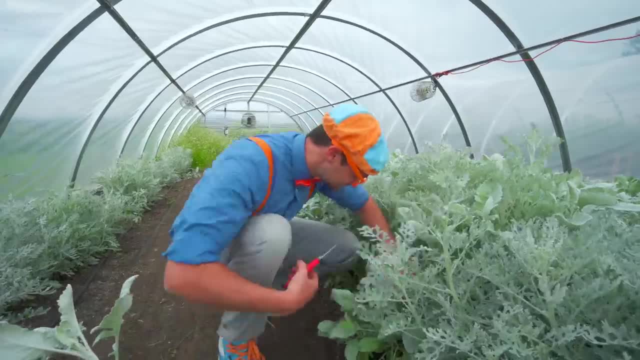 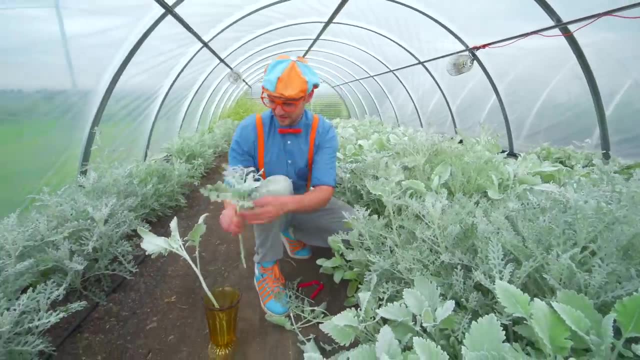 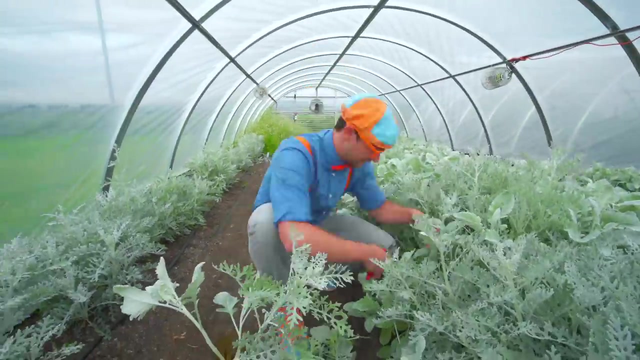 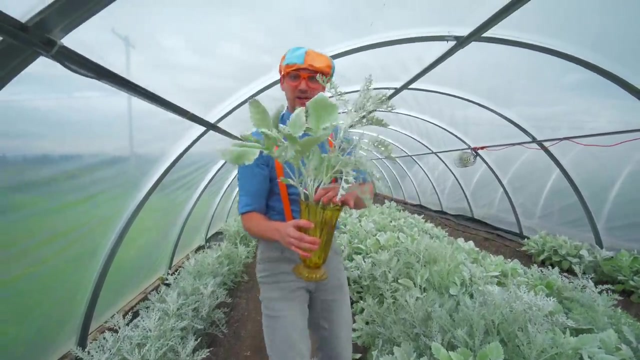 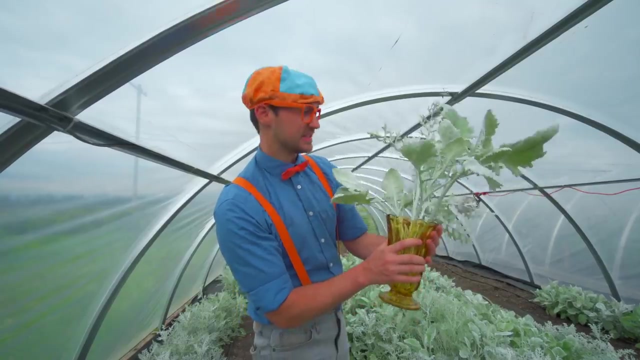 All right, Let's cut some more, shall we? There we go. All right, Perfect. And some more. All right, Let's make a bouquet. Whoa, Look at all of them. They're so beautiful. All right, what else do we need? 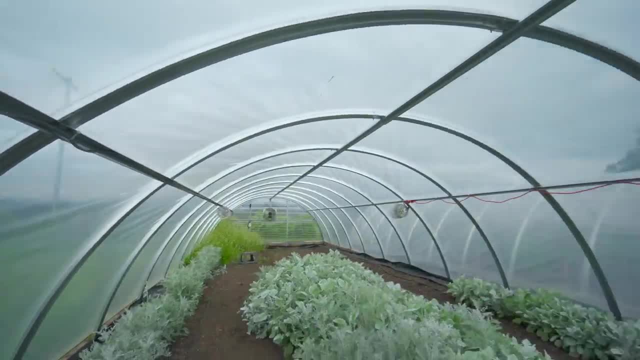 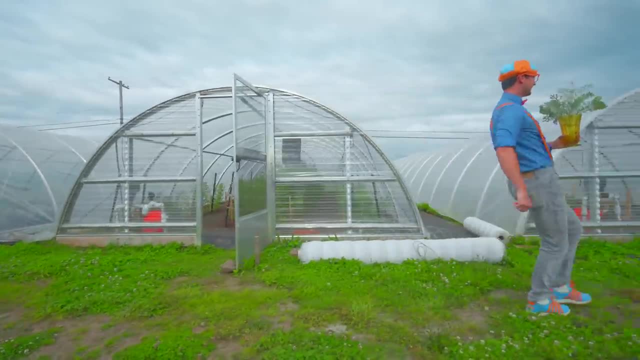 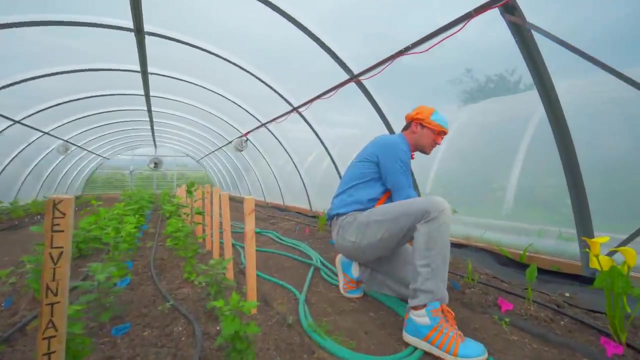 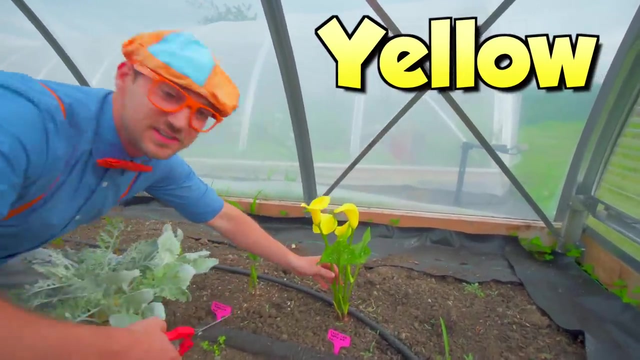 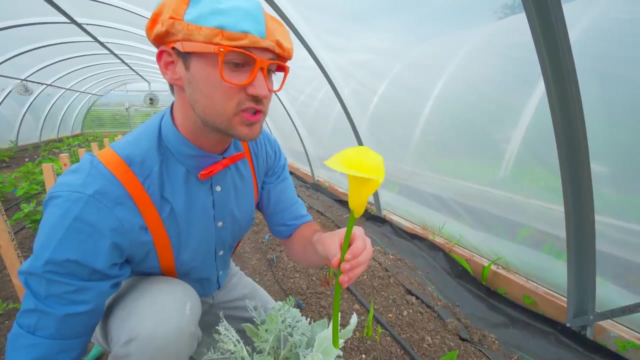 We got a nice base. We need some color. Let's go. Oh, look at these colorful flowers. Yeah, they're the color yellow. These will look beautiful in the bouquet. All right, Whoa, so interesting looking. Okay, let's put that right there. 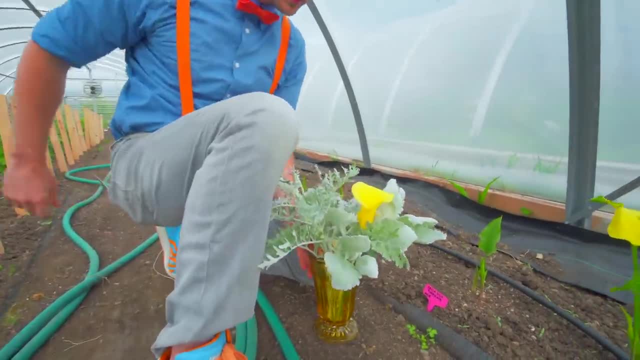 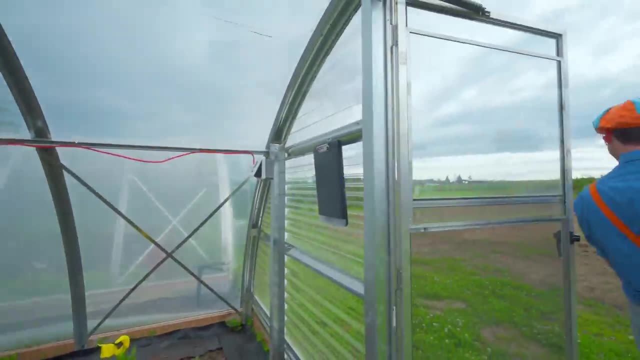 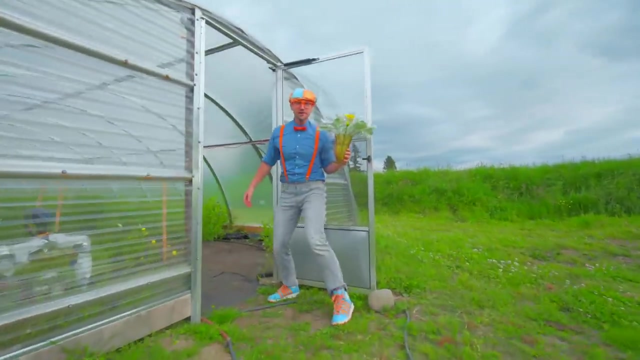 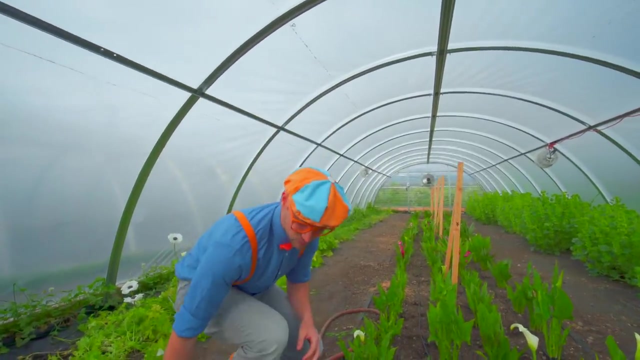 All right, one will do. Oh, all righty, let's find some more flowers. Come on, Oh, another growing room and more flowers. perfect, Just what we're after. All right, look at this one, huh. 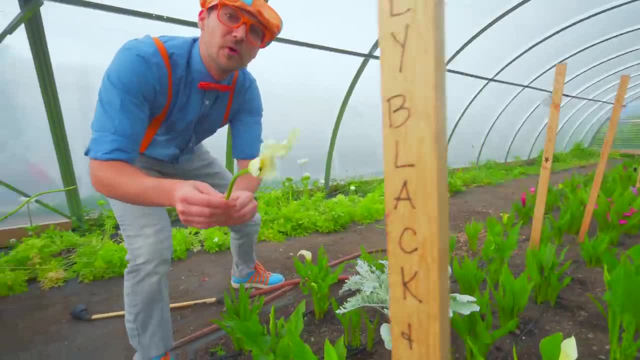 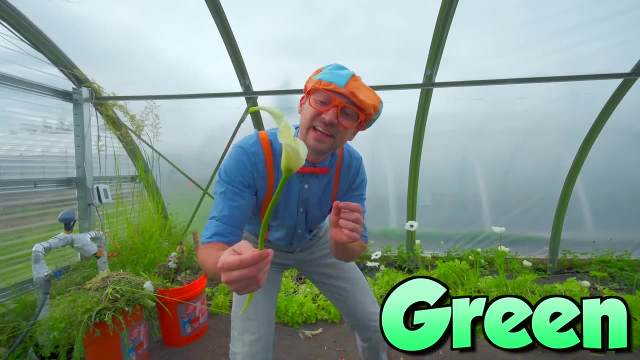 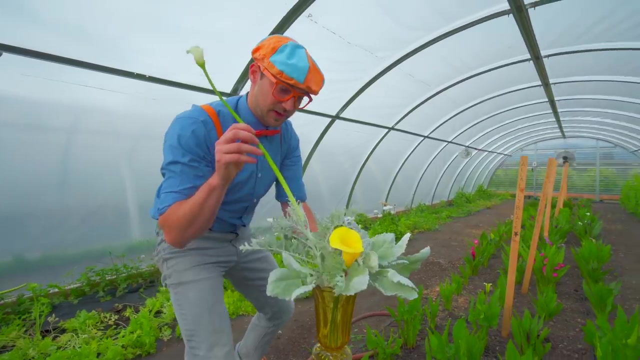 All right, let's pull it up. Ooh, it's kind of white. Yeah, it also has a little bit of green and a little bit of yellow. Yeah, and it makes that color. All right, let's put it right there. 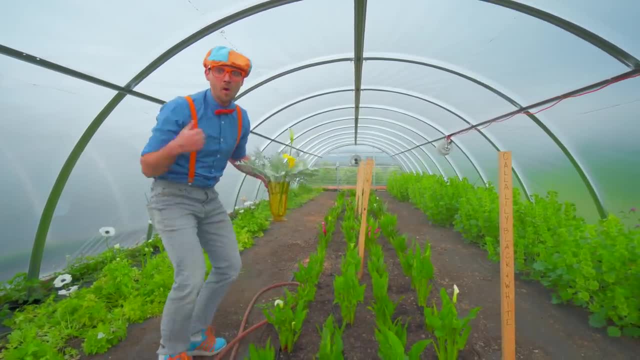 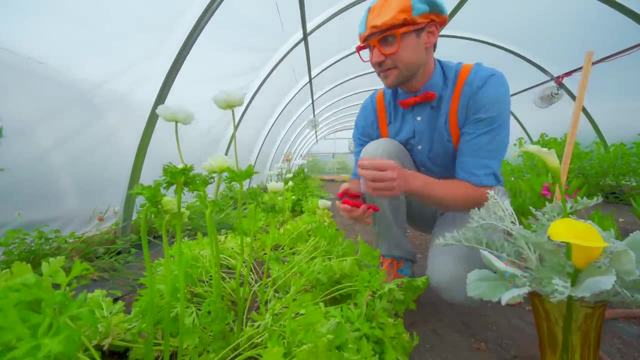 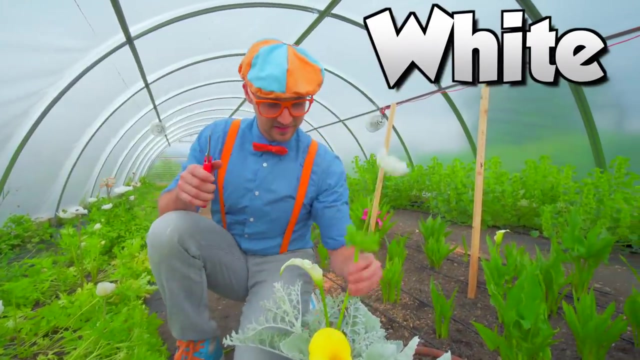 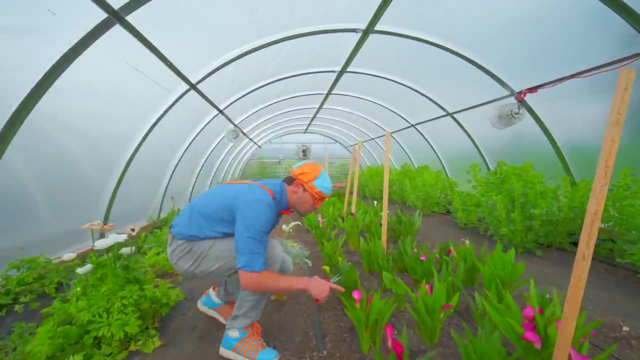 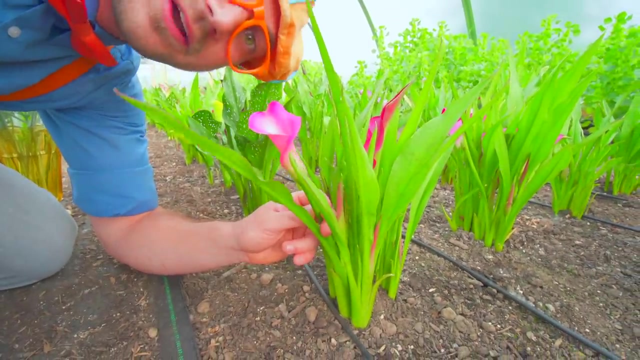 Yep, perfect. Oh look, Wow, take out our scissors. Gotta be careful, Okay, Ooh, that one's the color white. Put that right there. Ooh, Whoa, look at this one. Yeah, this color is the color pink. 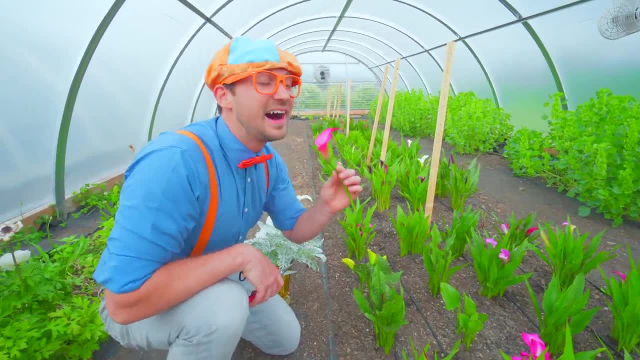 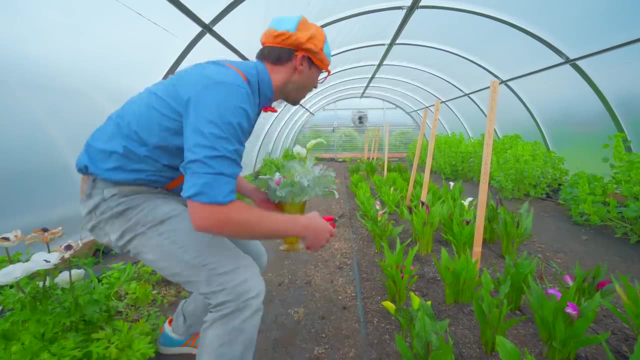 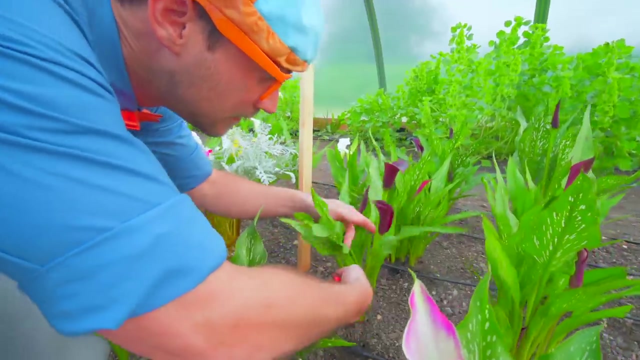 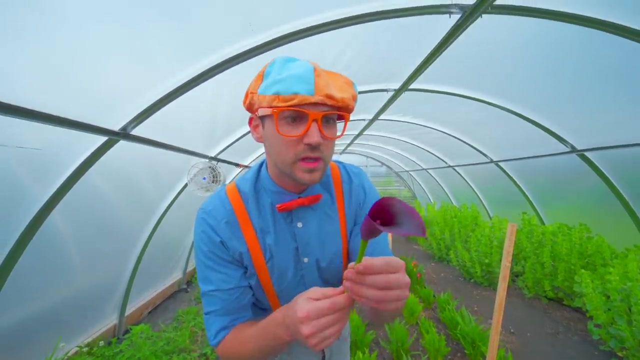 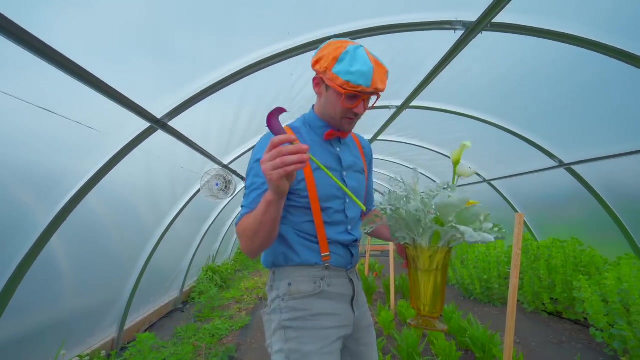 Wow, so beautiful. Ah, it smells so fresh. All right, and one more over here. Whoa, Whoa. look at that color. Whoa, it's a really deep, deep, dark purple Whoa, that will look beautiful in the bouquet. 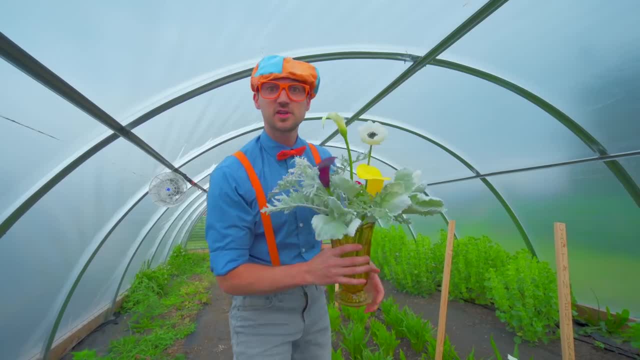 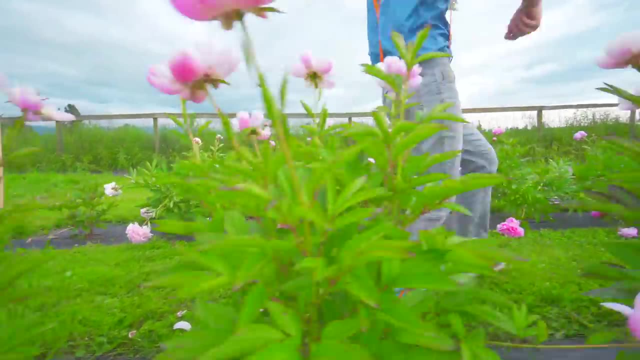 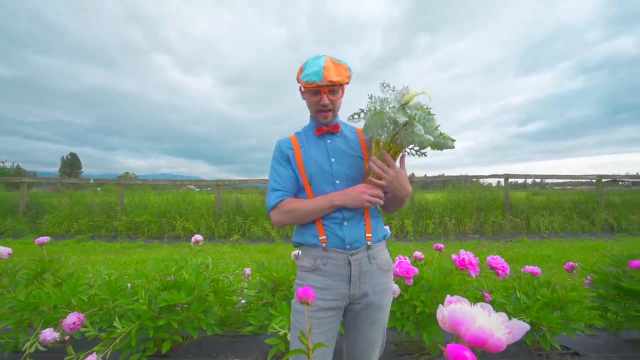 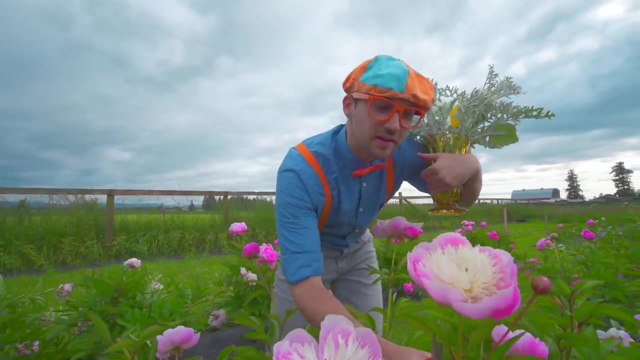 Let's put it right there. All right, Let's go find some more flowers. Whoa, Here's some more beautiful flowers for a bouquet. All right, let's take our scissors. Be very careful. This one looks perfect. Actually, this one looks perfect. 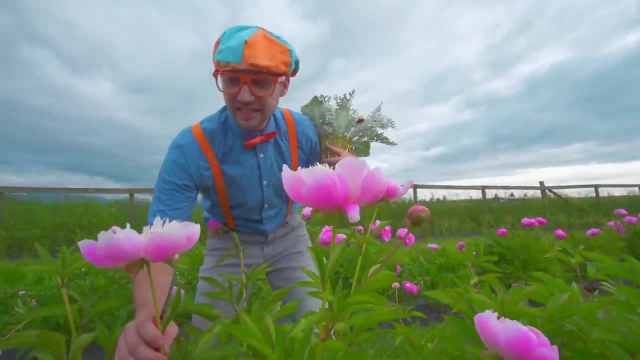 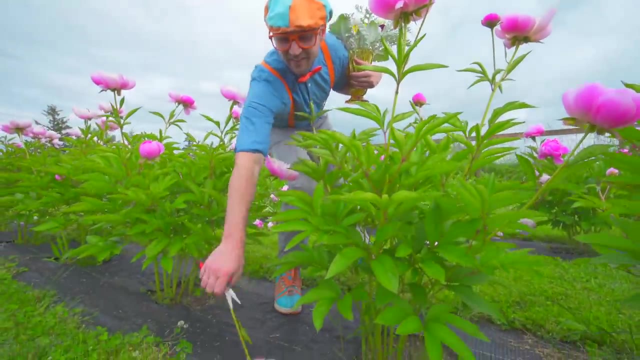 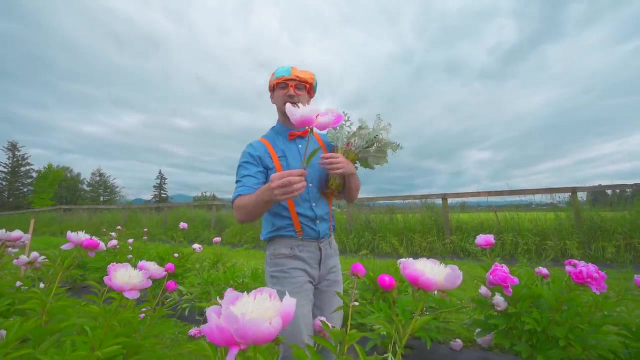 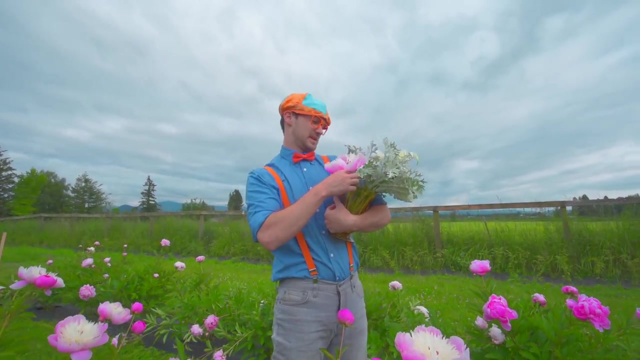 See the color. It's the color light pink. All right, Oh ha ha, It fell. All right. All right, My snippers back there, All right, ah, Oh, So beautiful. All right, put it right there. 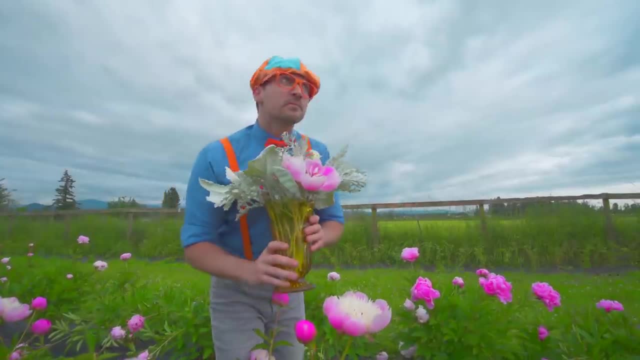 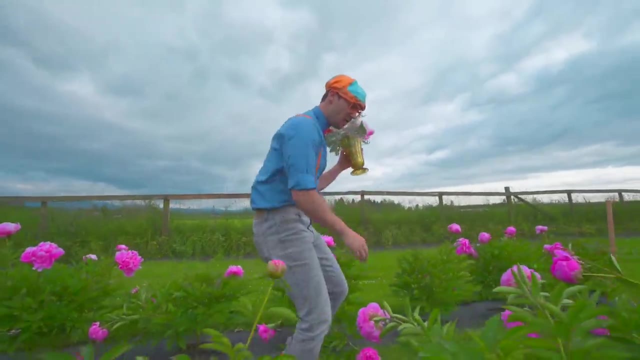 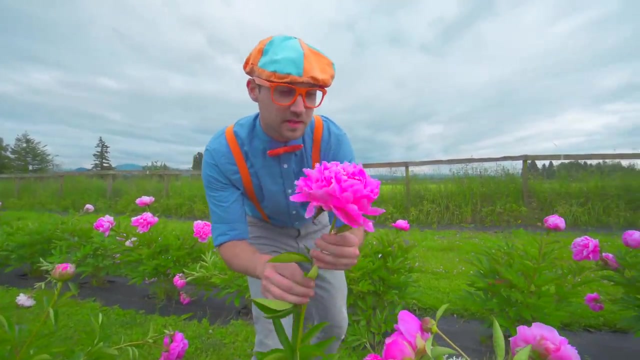 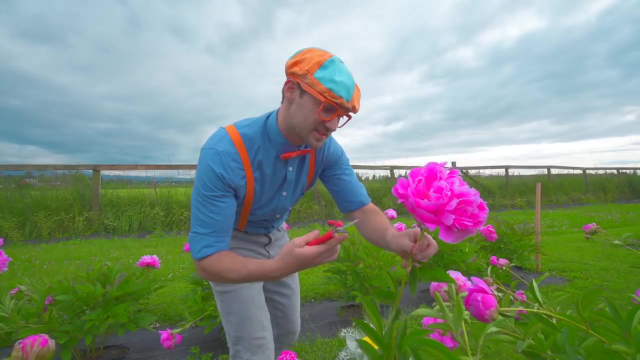 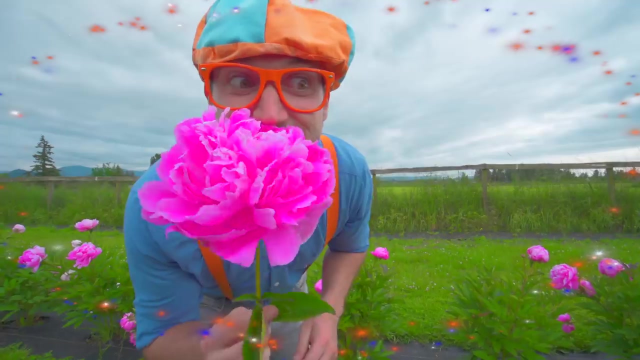 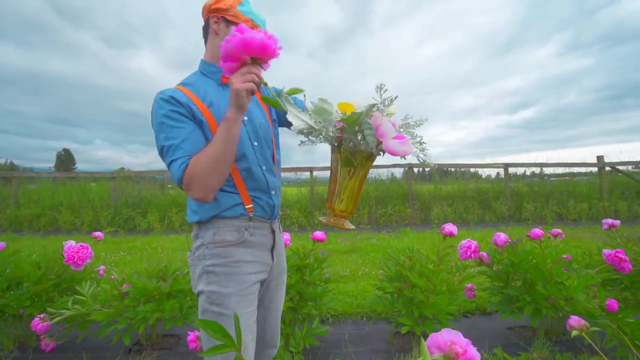 Whoa. look at it now And it smells even more beautiful. okay, whoa, some more flowers. all right, this one looks ready and this one is dark pink. Wow, all right, let's take the scissors, give it a snip, give it a smell. mmm, so fresh. all right, here we go put it right there, whoa. 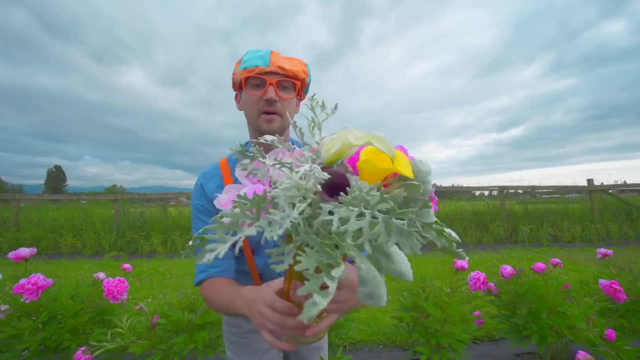 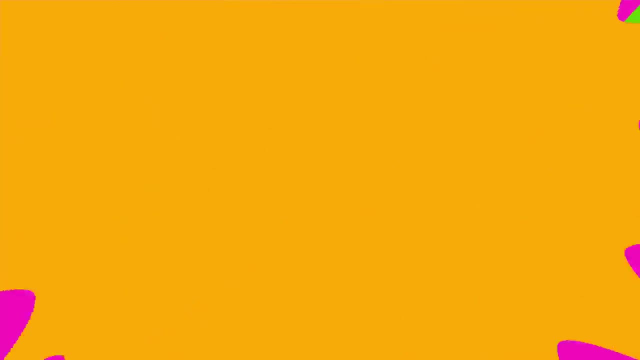 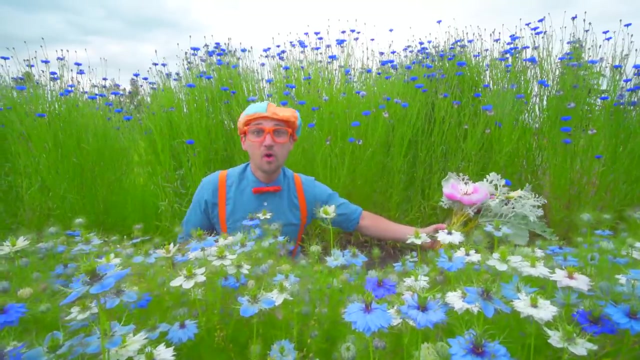 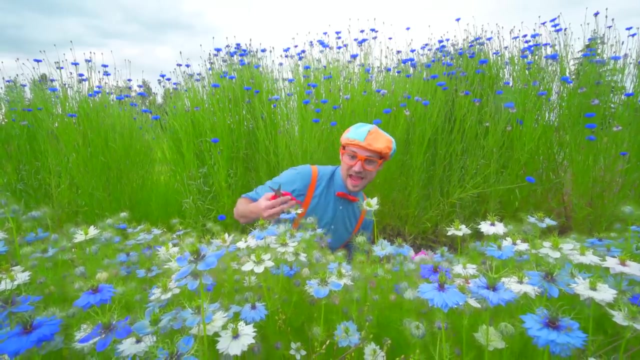 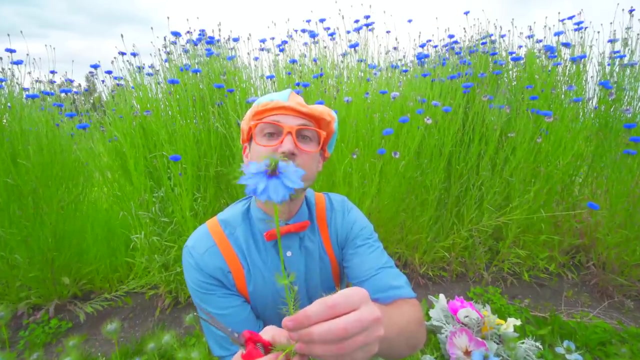 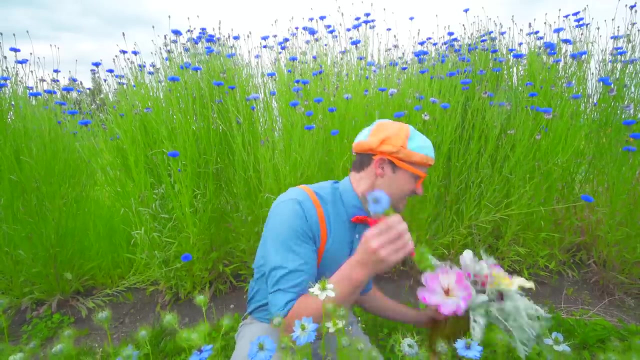 that's a big flower, whoa, it's so colorful. oh, I see some more over there. haha, more beautiful flowers for our bouquet. all right, let's cut some flowers together. all right. whoo see this flower. this flower is the color light blue, Wow, beautiful. all right, let's put it in here. all right, perfect, all right, let's. 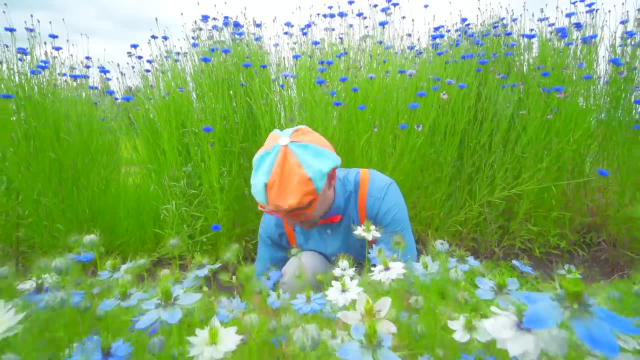 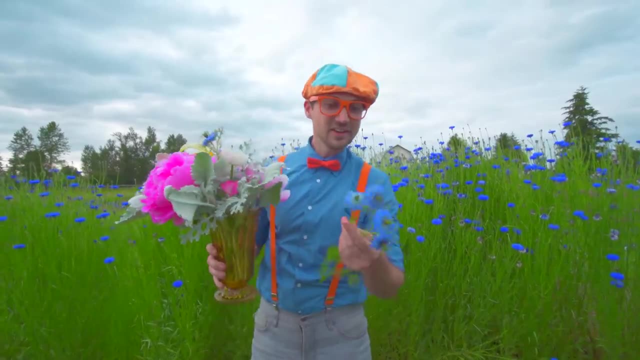 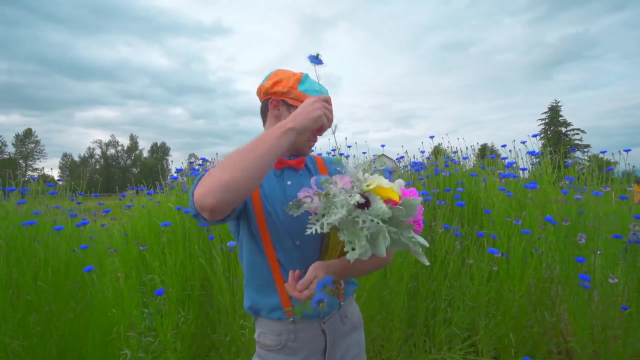 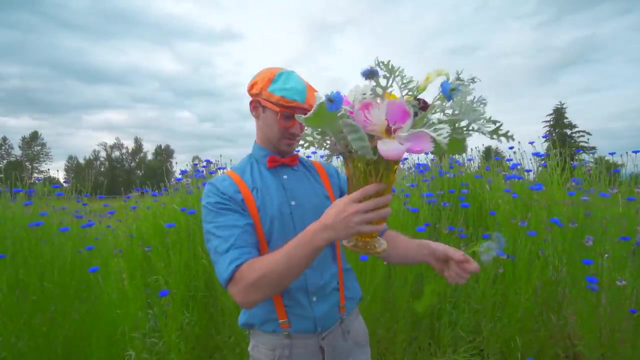 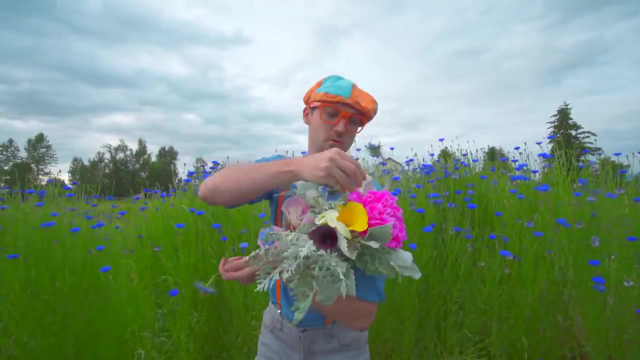 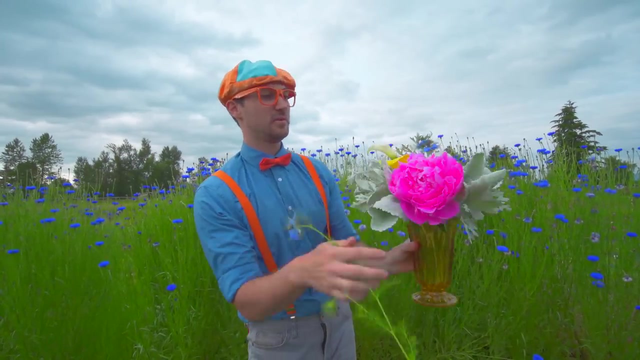 cut some more. here we go, you all right. look, we have some more to place in here. about one right there? how about one right here? and we have two more? one, two, two, two, five. Let's put one right there, perfect. And let's put the last one right next to this big one. 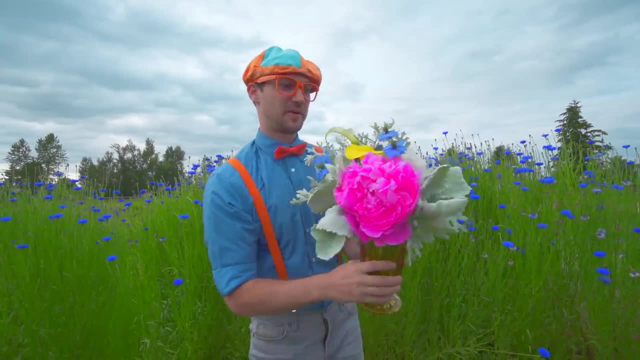 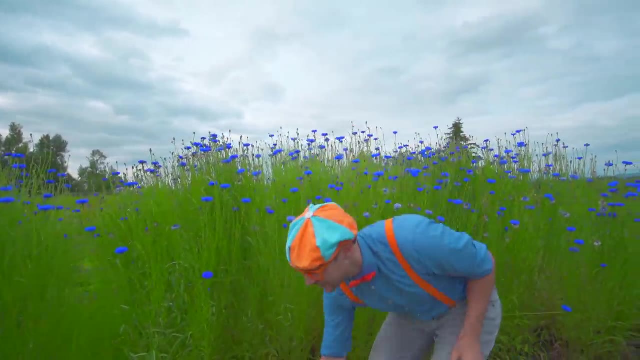 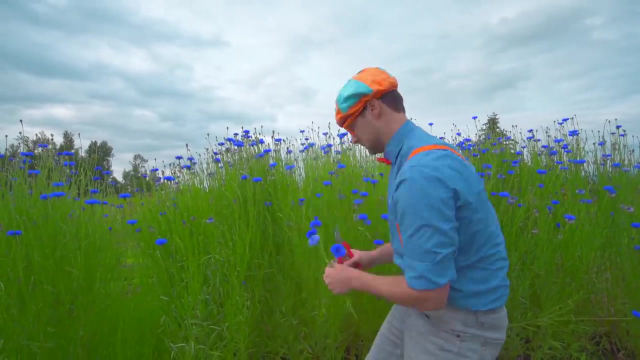 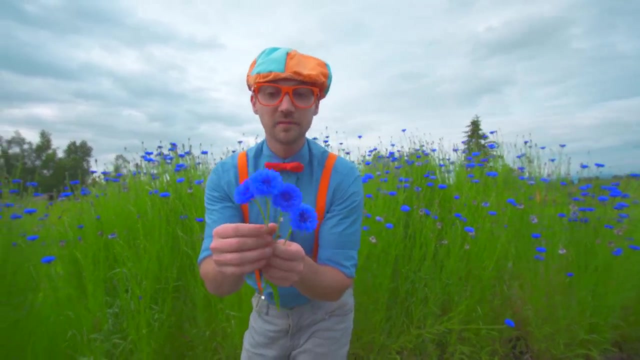 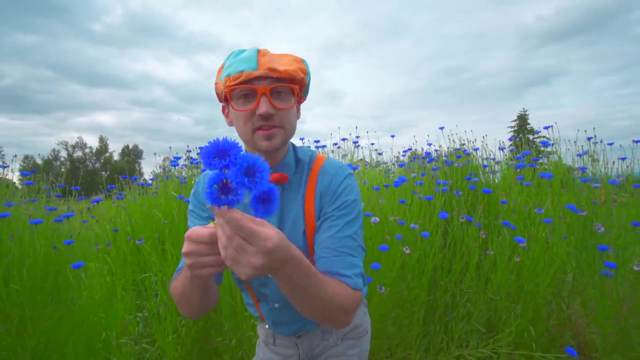 All right, there we go. perfect, So beautiful. oh, look more blue flowers. All right, let me snip some of these. Huh, these are the color blue as well, But remember the last flowers? They were light blue, but these flowers are dark blue. 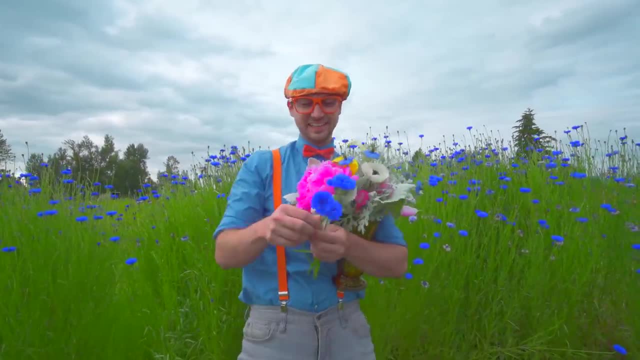 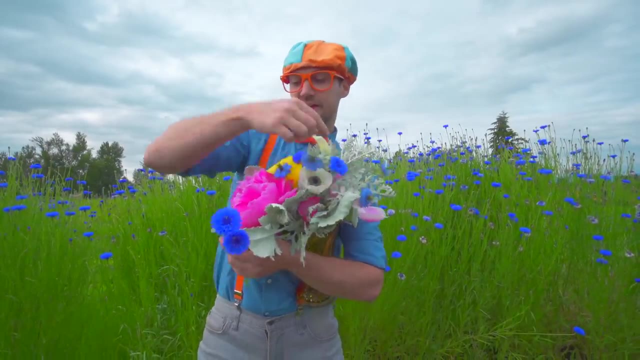 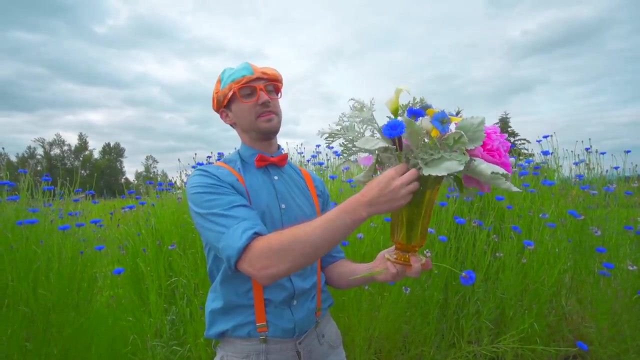 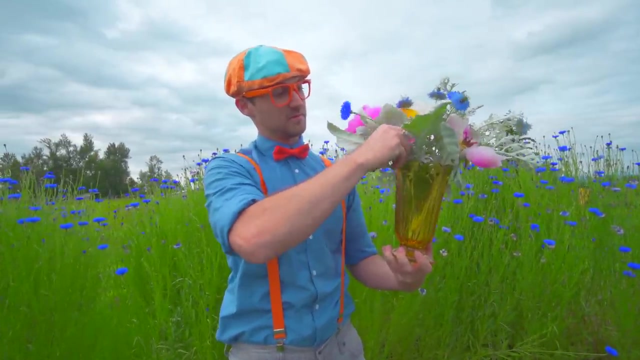 Let's put them in the bouquet. all right, here we go. How about one right there? how about one over here? how about one? One? let's see, right there, looks beautiful, And one right there. whoo, what a beautiful bouquet. 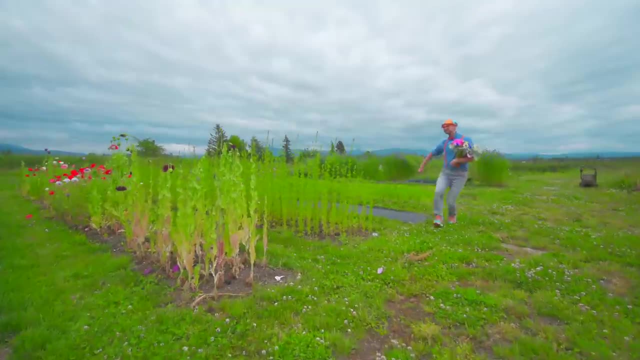 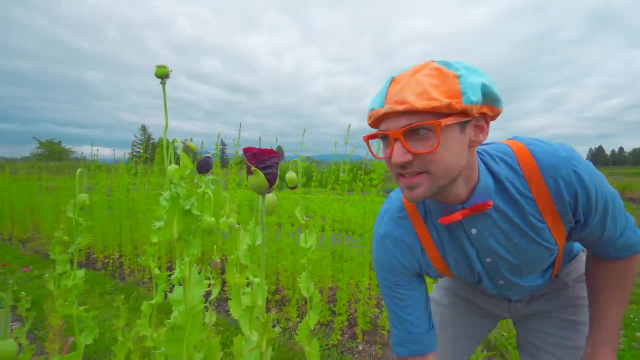 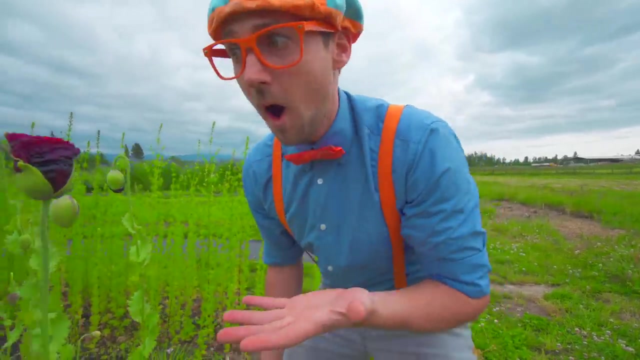 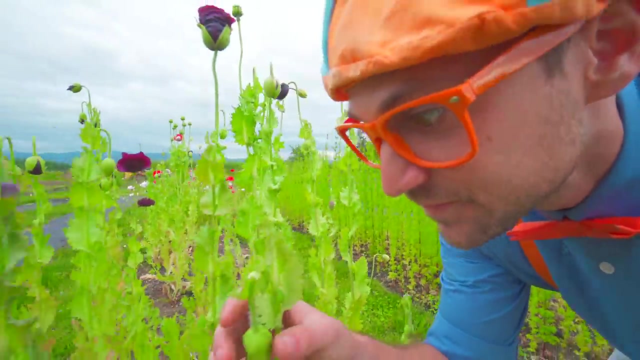 Let's go get some more flowers. Ooh, some more flowers. ooh, interesting. See this flower. It's not fully blossomed yet. huh, yeah, ooh, There's different stages of blossoming flowers. Look down here. see. this one hasn't even opened yet. 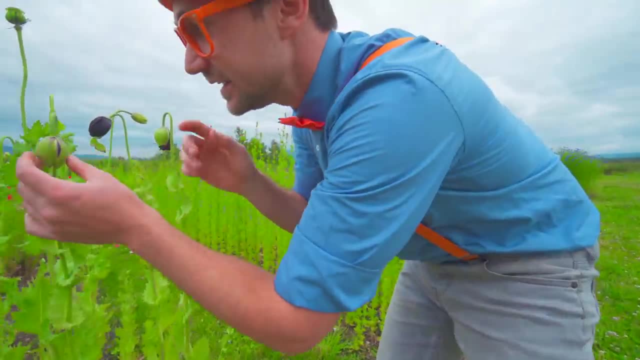 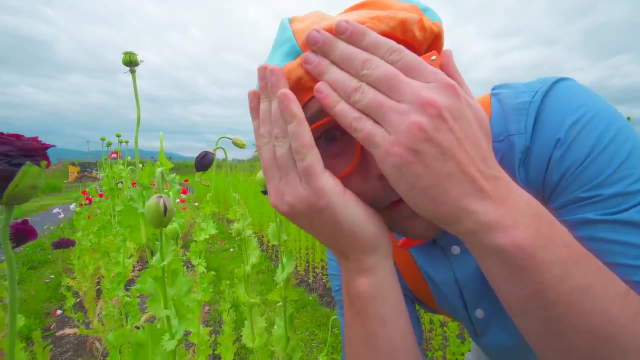 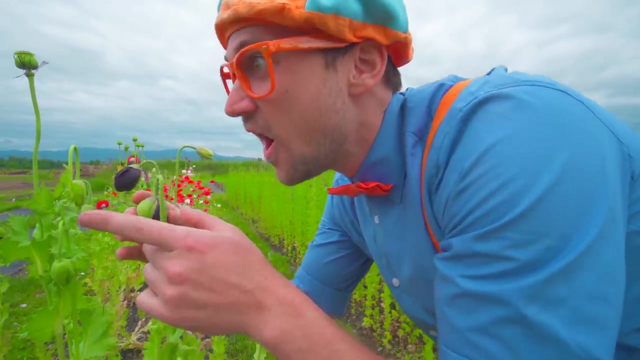 It's still a baby. ooh, you see this, It's trying to peek out. it's like hello, I see you. But then it opens a little bit up, a little bit more see, And then goes to a little bit more yeah. 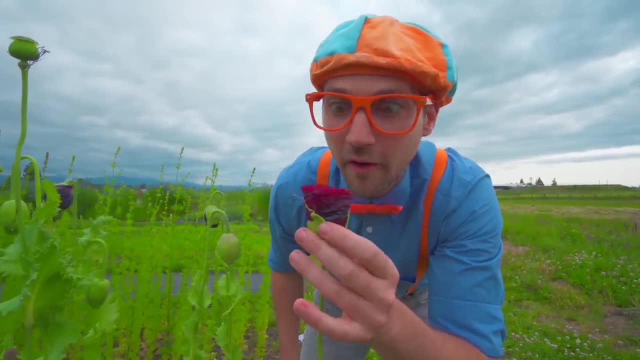 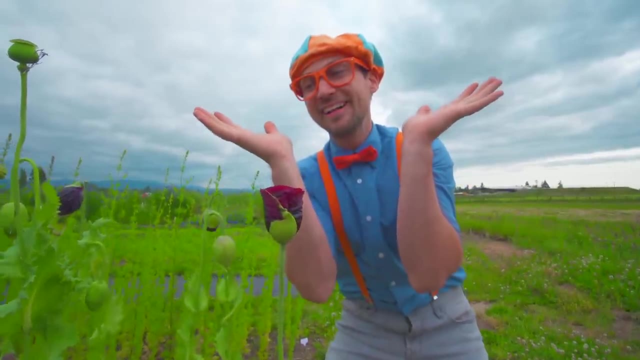 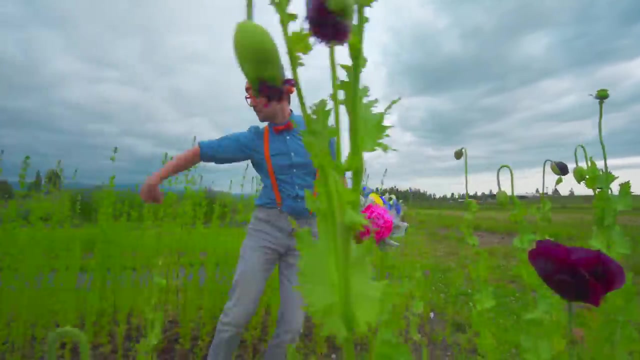 And then goes even more whoa. And then, after that goes: whoa, I'm beautiful, I'm a flower, And speaking of that, there's some down here, let's go. Whoa, look at these whoa, let's cut one. 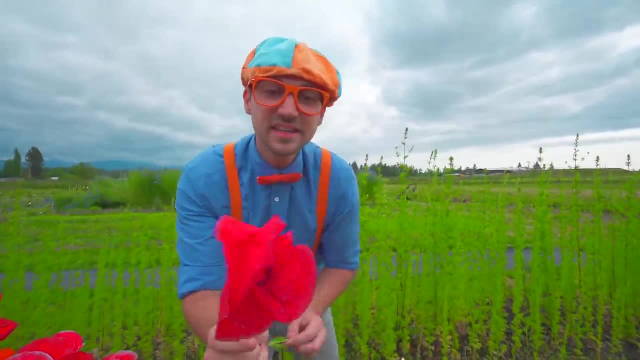 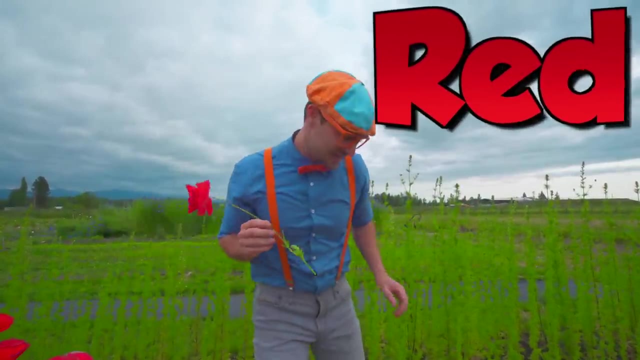 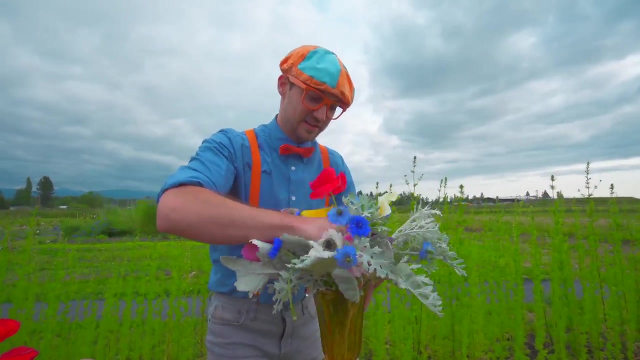 Whoa, this is a new color, do you see it? Yeah, this color is the color red. All right, let's add it to the bouquet. Let's put this one right in the very, very center. Whoa, look at that, it is so beautiful. 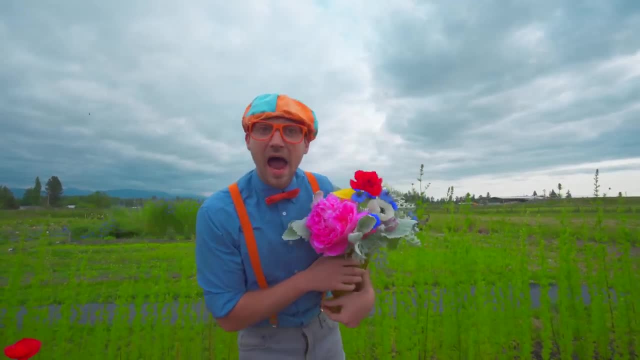 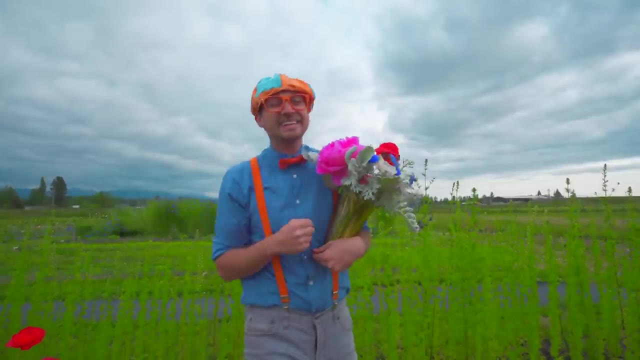 I know what I'm gonna do with these flowers. I'm gonna surprise my mom. Shh, if you cut flowers, you can do the same. Well, this is the end of this video, But if you wanna watch more of my videos, 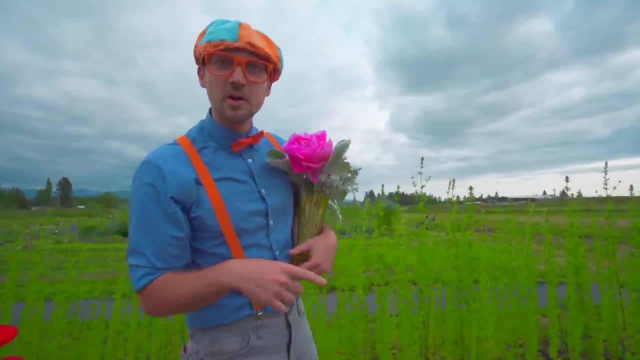 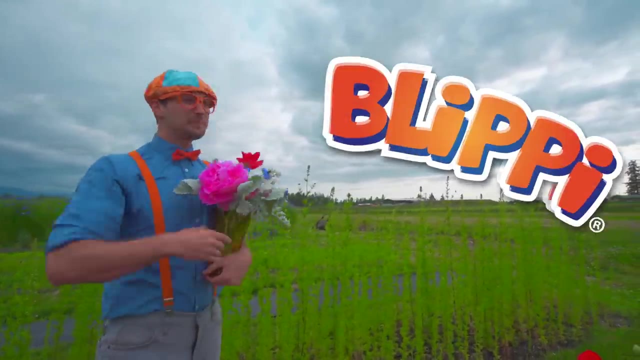 all you have to do is search for my name. Will you spell my name with me? B-L-I-P-P-I, B-L-I-P-P-I, P-P-I, Blippi, Good job, all right, buh-bye. 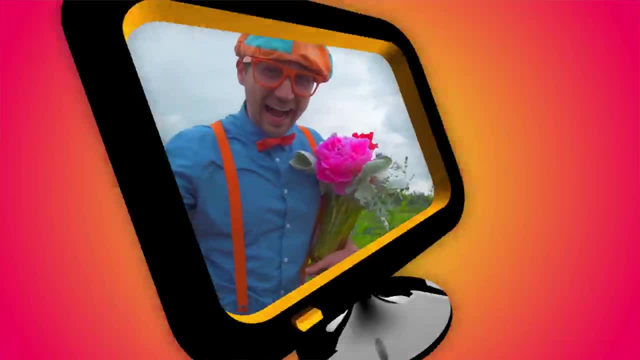 Love you, mom. So much to learn about. It'll make you wanna shout Blippi. 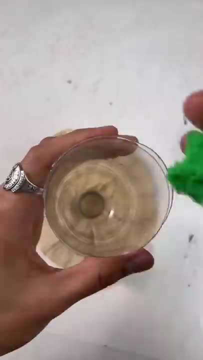 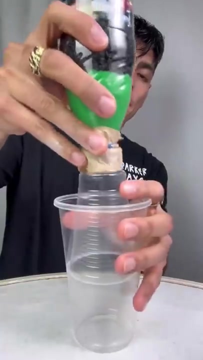 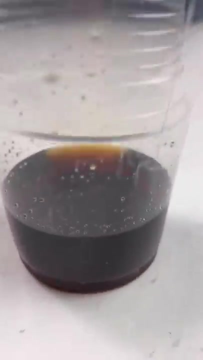 This helped me get an A in third grade. Let's pour some soda into it. Okay, so it didn't filter out the color, but let's see if it filtered out the sugar. It got rid of the fizziness. Let's confirm if there's any sugar in it. 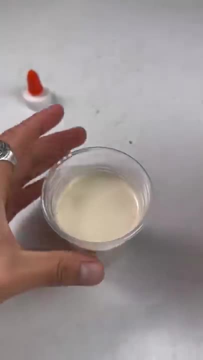 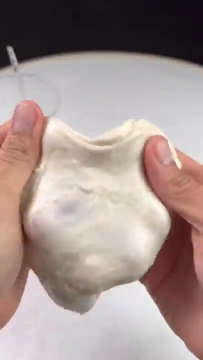 If this works, at least the sugar was filtered out. Mix it up, Let's add some borax. If it doesn't activate, there's still sugar in it. Okay, it activated. It worked A little over activated, but it did come out pretty good.